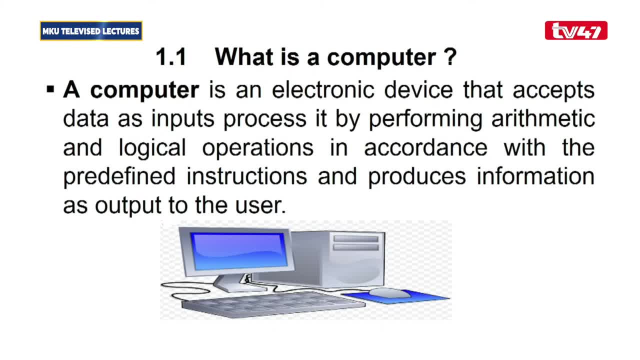 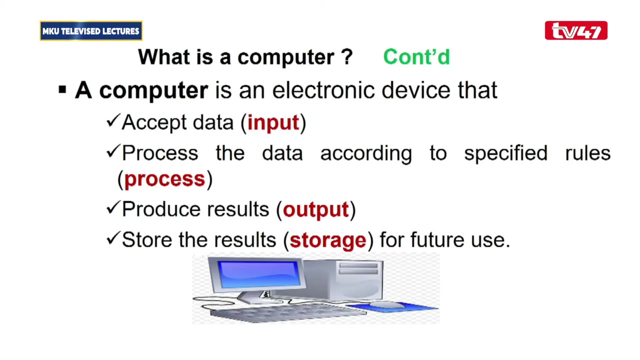 that input, through the central processing unit, based on the predefined instructions, to produce information as output to the user or to be taken to the storage for the computer. So a computer is a system that is made up of those four major components. It's made up of the input devices that takes up the input from the user, which is in form of raw. 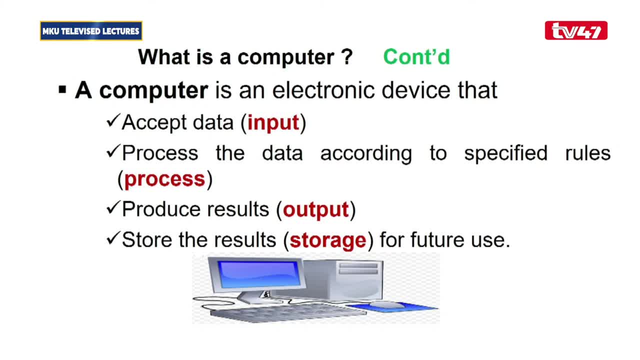 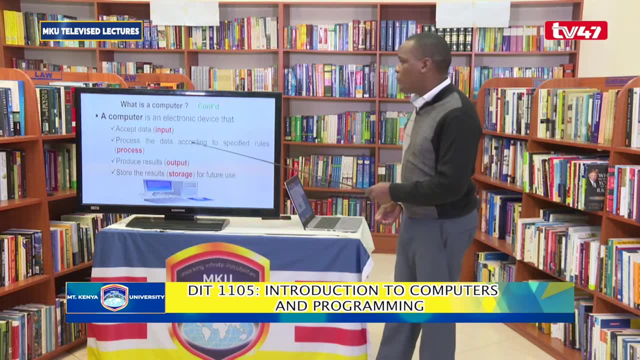 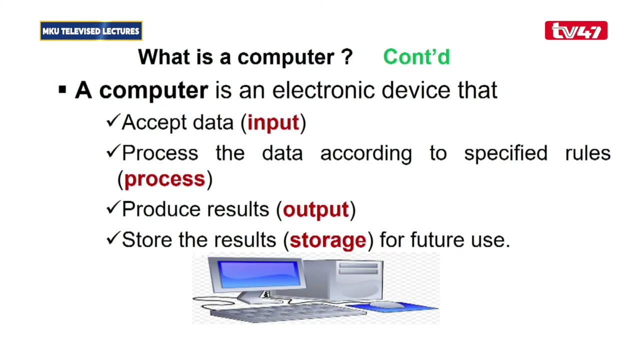 data or variables that are not processed, which are taken to the processor for processing, And this is where we have the central processing unit. So a computer is a system that takes processing unit, that processes these data into information which is taken to the user in form of an output. and this output, which is informal information, can 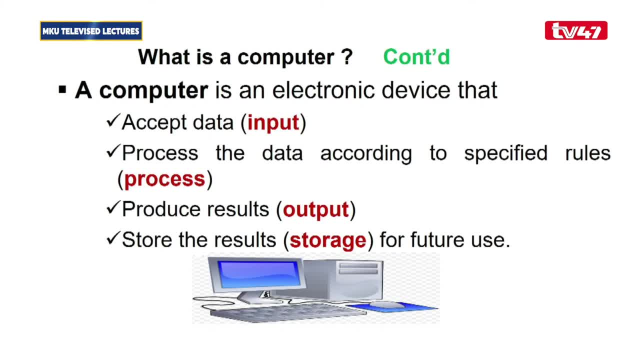 be taken to the storage, the storage unit. all they can be displayed on the screen to the user. and these four component are the key areas that makes up a computer. we have other electronic components or electronic devices that do not qualify it to be a computer, like the television, the radio, the mobile phones and other. 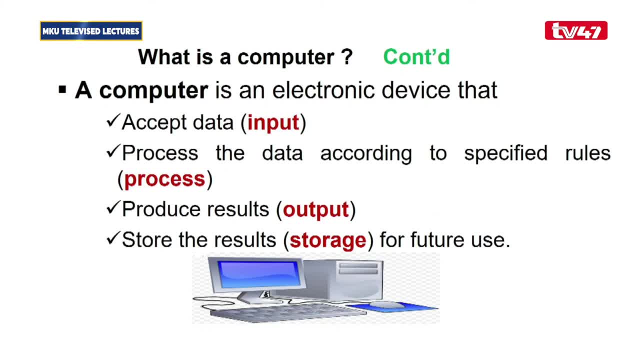 electronic components that exist because they do not perform these four major areas. you fight like a television and or the radio may perform one or two of these areas, as much as it is an electronic device, but a computer performs all that, these four areas. and therefore this: what qualifies or makes an electronic? 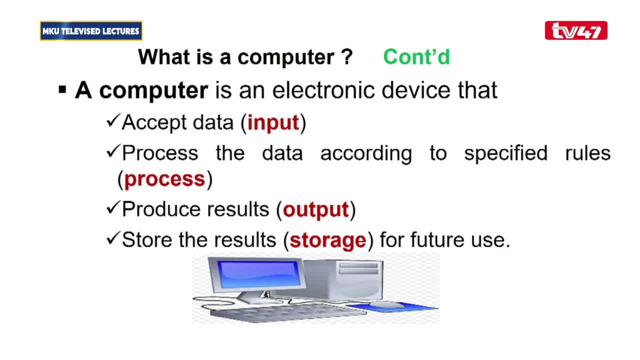 component to be a computer and each of these component has various devices that works alongside with it, like in the input device. there are quite a number of input devices that exist that the user can use to enter data into: the keyboard, the mouse, the microphone- all those are input devices that 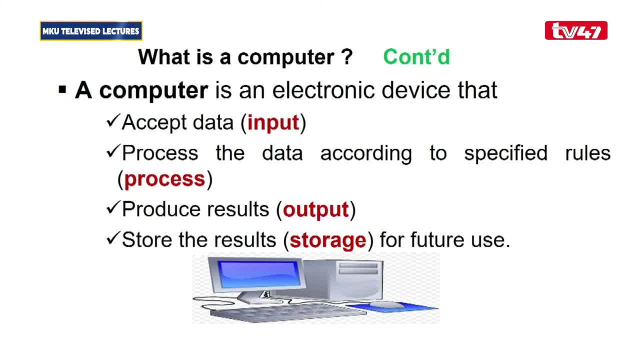 the user can use to accept data into the to the computer. the processing is done through the processor and then on the output again. we have quite a number of output device, depending on what the user enters in here. if you enter sound, then the output will be in form of a speaker which will produce that particular sound. 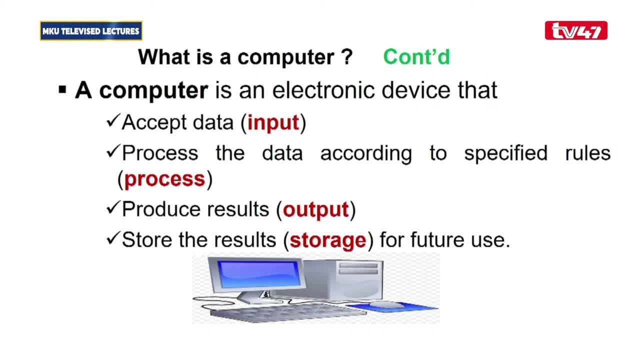 if it is digital data, the screen will be an output device for that particular matter, and the output again can be in form of a printer. it is a hard copy and the data can be stored into the internal storage of the computer or external storage, where we have the external storage devices. 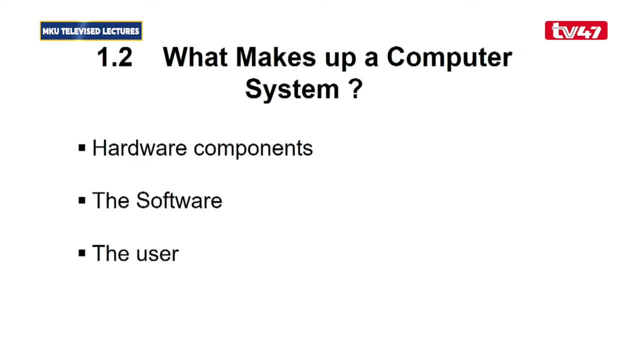 that what makes up a computer. again, a computer is a system, meaning that it is made up of several components that work together, which means a computer with a single device. if you put uh a computer, you can ship computer. or​ if you have 5 or 6 computer, if in practice you can receive chopped or procu propositions on that computer. if it's not Truly a computer, 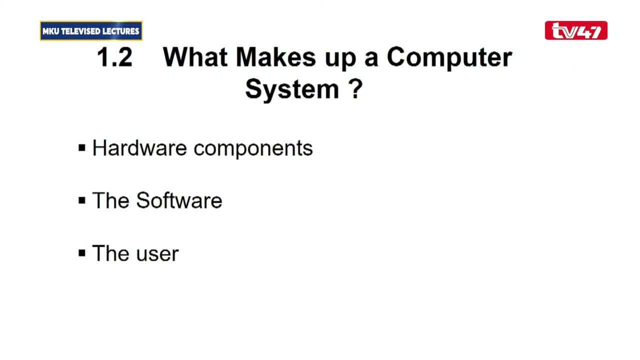 work together as one, they work together as a unit. So we have the hardware components, the software components and then the user or the people who are using the computer. The hardware components are the tangible parts of the computer, the physical parts of the computer, which includes the keyboard. 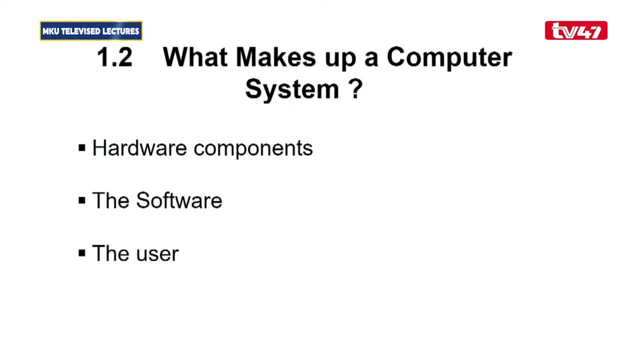 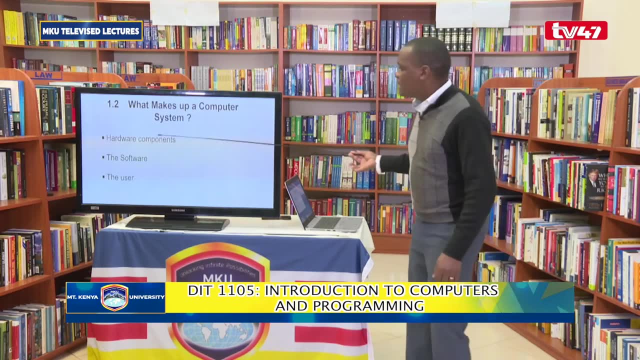 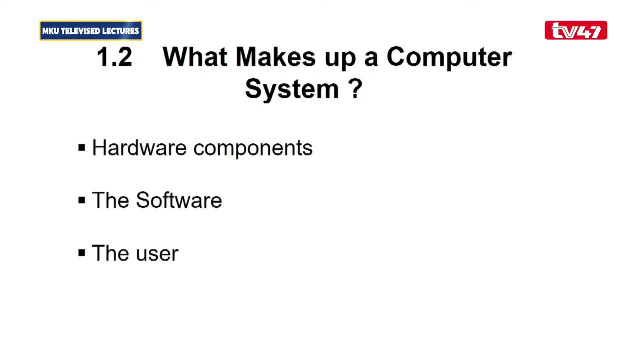 the mouse, the screen or the monitor, the hard disk, the processor, the motherboard or the physical parts of the computer. There are quite a number of them. They are categorized as hardware components which cannot work on their own. They require programs or softwares to control them. 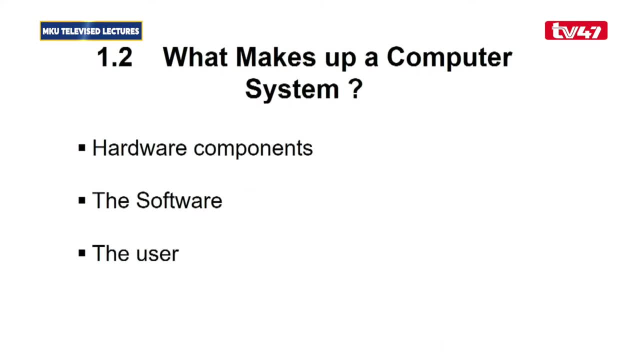 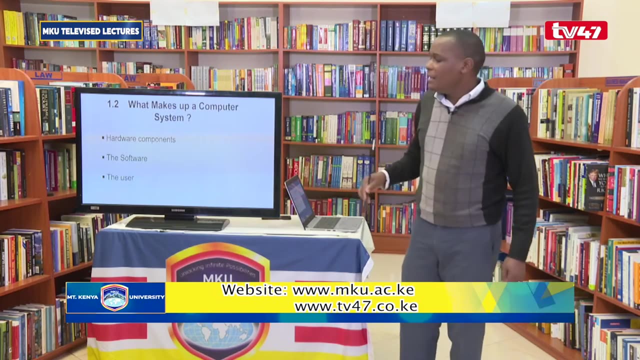 And softwares are a set of instructions that control what the hardware components does, And this is done through the user. The user is the one who feeds the commands that get through the software, The software to control what the hardware does. So we have the users of the computer or the person controlling the computer. 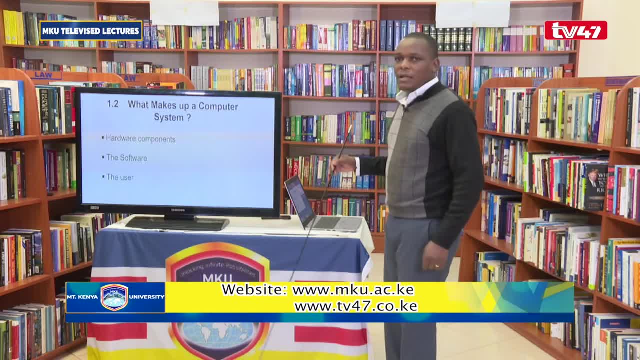 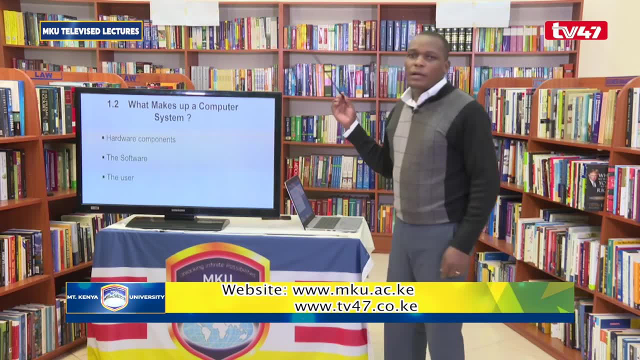 For instance, the user may want to save a document. To save a document, that command- save command- is activated by the user Who clicks on a particular point of the screen or particular point of the application program. Let's say you're using Microsoft Word- which will prompt that command to. 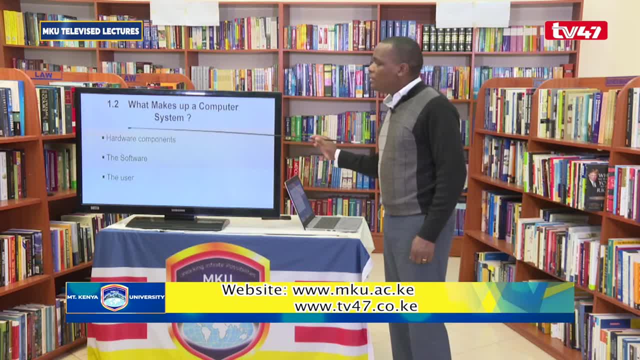 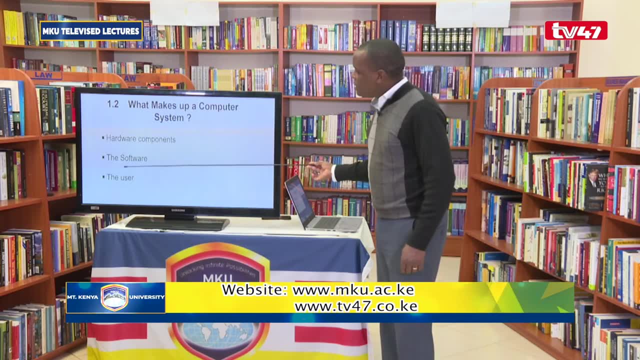 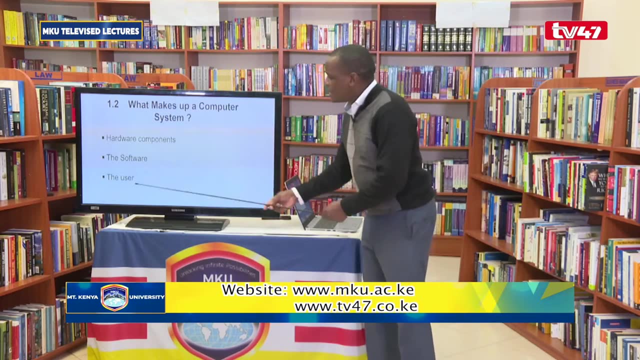 save or to move that file to the storage unit. Maybe you're saving it on a flash disk or a hard disk or any part of the computer And therefore the user drives that command that the hardware acts on, And these three works as a unit. 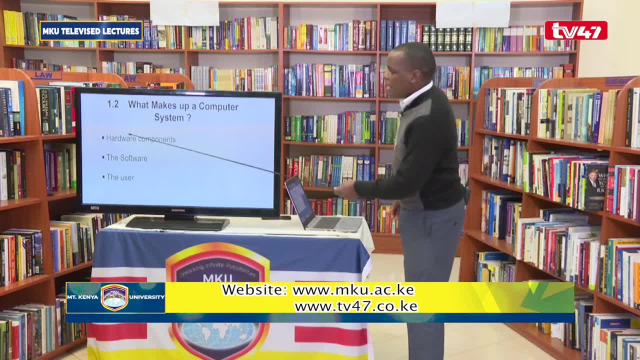 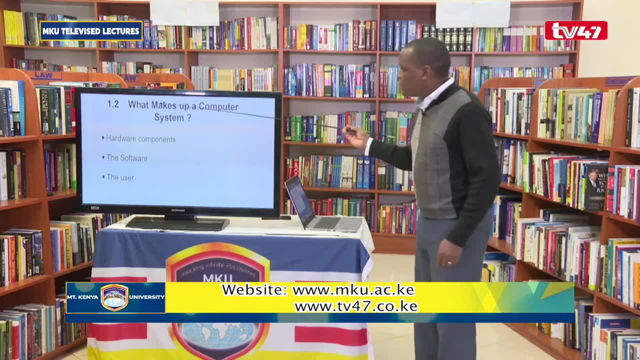 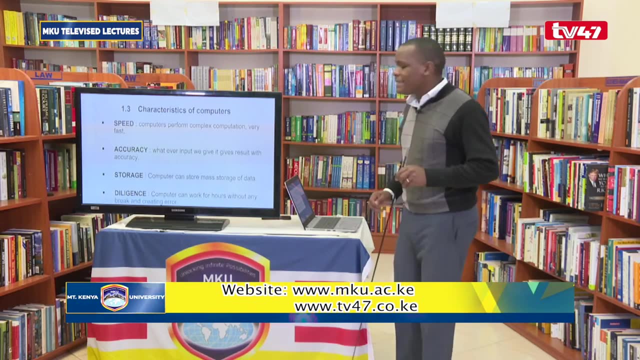 Therefore the hardware cannot work on it on their own. The hardware and the software cannot work on their own. They require the user to control and drive them. Therefore the computer is referred to as a computer. Then this particular computer has a number of characteristics. that makes it suitable. 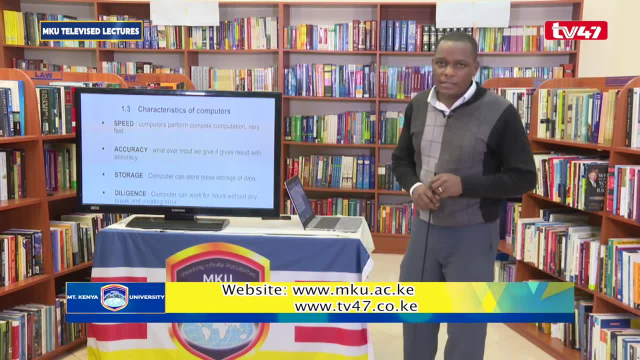 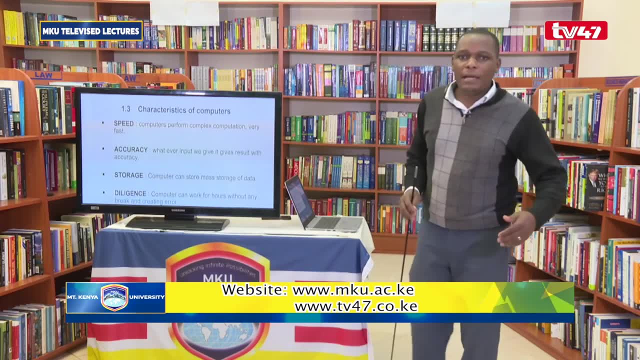 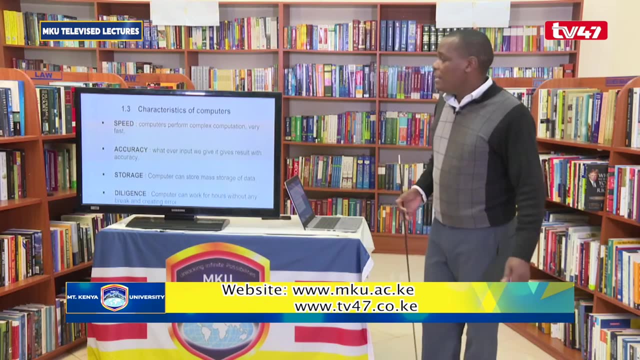 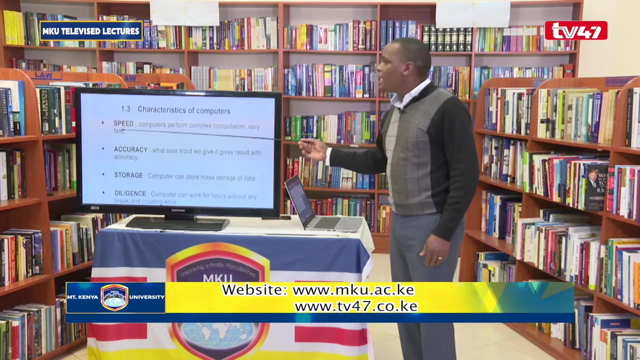 especially in the application areas that we use computers, Because before computers came about, the same tasks they are performing were done by human beings, And what makes the computer better in particular specific areas is because of some of their characteristics, For instance, when it comes to speed, they can perform complex calculations and computations. 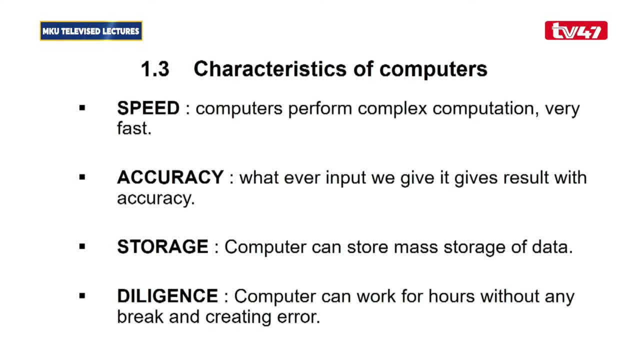 within a matter of seconds. What a human being would take more time? like when you're multiplying a million times a million times a million. the computer will do that within a microsecond, But a human being might take a minute or two to do the same. 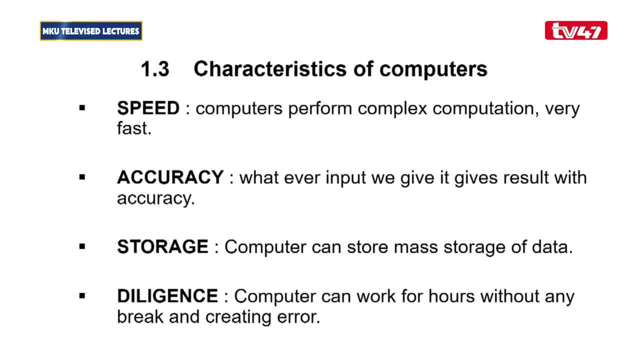 Therefore, they can be able to perform a lot of tasks and complex computations within a matter of seconds. They are accurate based on the kind of instructions that you give them. If you give them the correct instruction, they will produce correct results. If you give them the wrong instructions, they will give you the wrong result because the 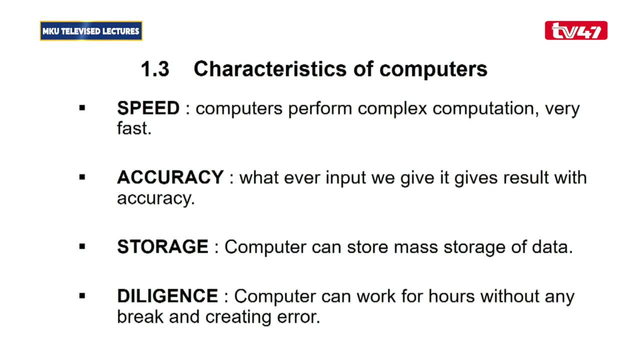 computer does not have the intelligence of their own. They depend on the kind of command the user enters in. They can store large amounts of data within a small space. They can store data in a small space, And they can store a large amount of data within a small space. 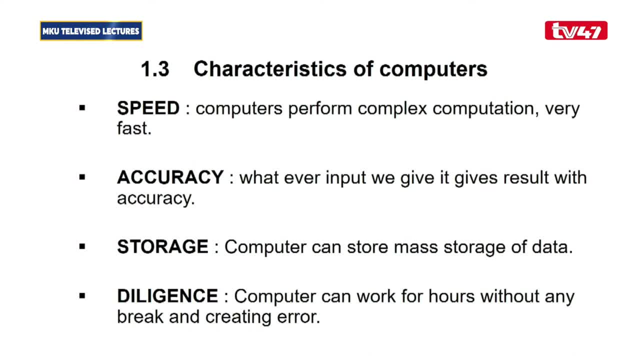 If you have a hard disk of one gigabit or one terabyte that can store large volumes of data, which would occupy a lot of space. if the same data was to be put in files in cabinets and put somewhere in an office, The entire office would be occupied with files. 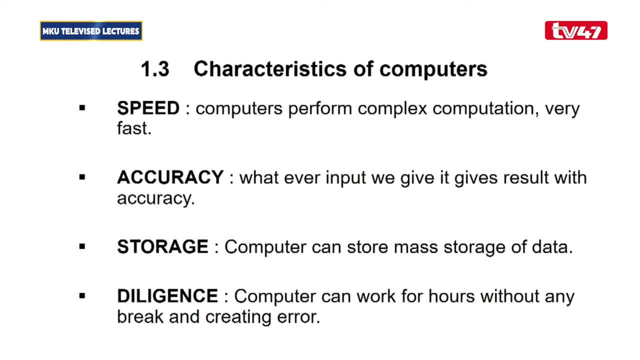 Compared to that, a single disk can store large volumes of data and therefore it makes them much better in terms of storage. Then they can work for many hours without getting tired, without complaining, without making an error due to fatigue, and so on. Therefore, diligence is also another characteristic of computers. 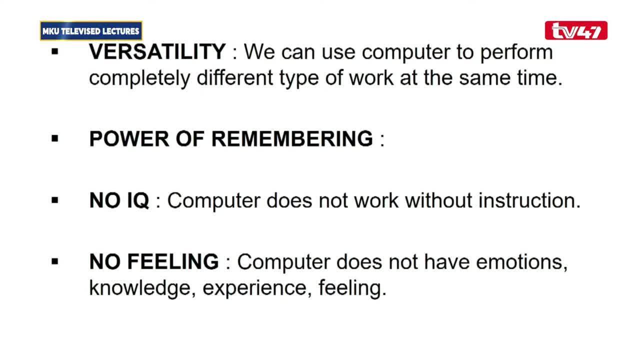 We also have versatility, where a computer can perform completely different tasks without complaining or without getting tired At the same time. in simple terms, they can be able to multitask, They can do more than one task at the same time, especially with the modern kind of software, the operating systems that support that. 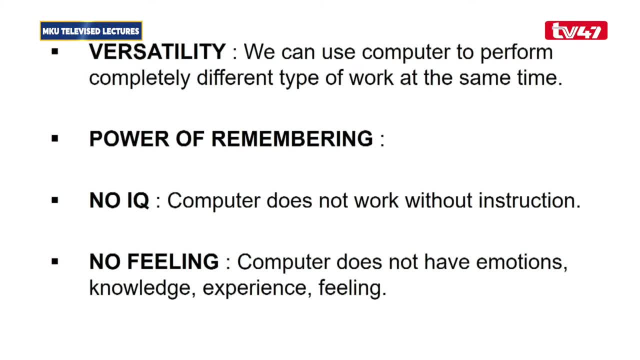 A computer. you can be using a computer. you are typing a document at the same time you are downloading a file from the internet at the same time. you are playing music using the same computer. At the same time you are printing a document using the same computer. 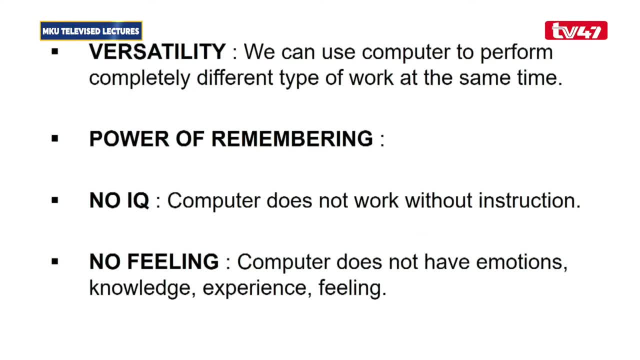 So they are able to perform quite a number of tasks at the same time. At the same time, due to the nature of the multitasking aspect of the computer, They also have a power of remembering. A computer can be able to remember quite a lot, especially the task that was done earlier on, compared to a human being, who may not be able to do that with accuracy. 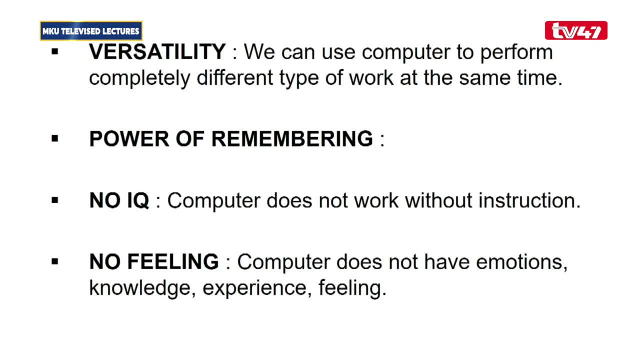 You can restore back to the computer to an earlier date, or you can refer back to a task that was done even five years ago, with accuracy And within a short time. So they have a power of remembering. Computers do not have intelligence of their own. 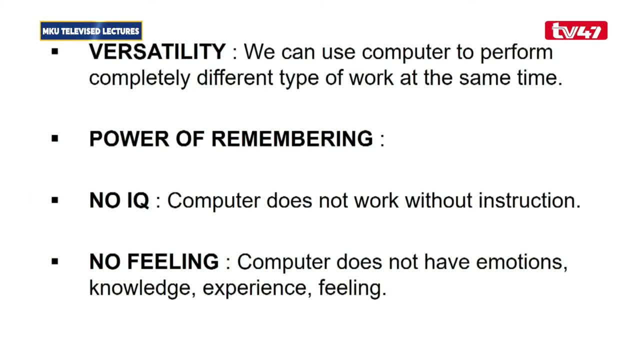 Therefore, they have no IQ or intelligent quotient. This is another characteristic of computers. Therefore, whatever you feed them is what you get out: Garbage in, garbage out, Meaning that they rely on the user's instructions to produce an output, And the accuracy and the correctness of the output depends on what the user does. 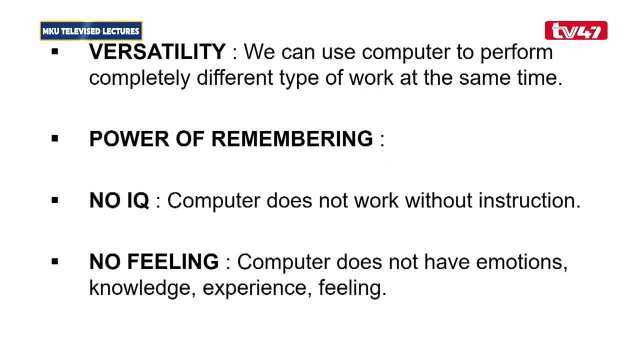 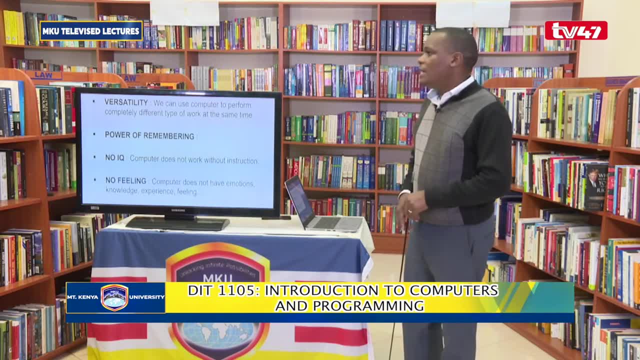 They have to have excitement at other people who are helping them. This is important. Usually, for example, when there are six or seven, Everyone on the computer is very quiet. Everyone gets into their computer. They have no feeling that. they do not have emotions. 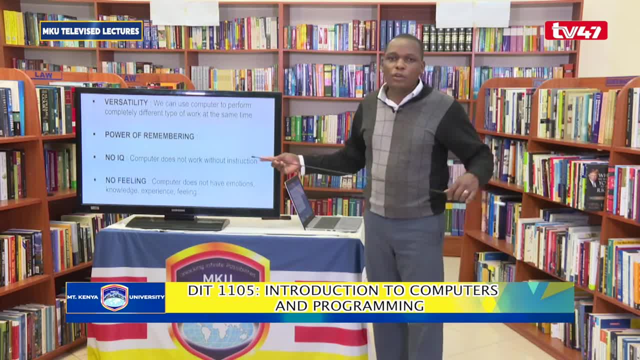 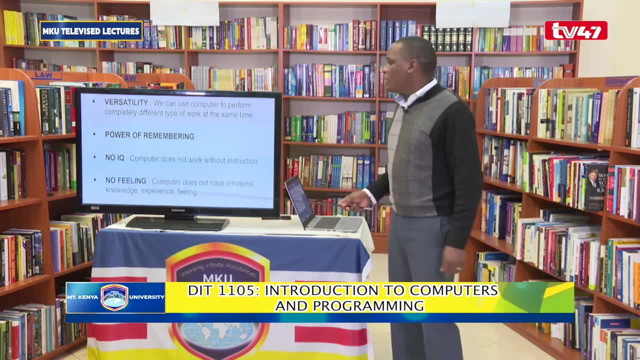 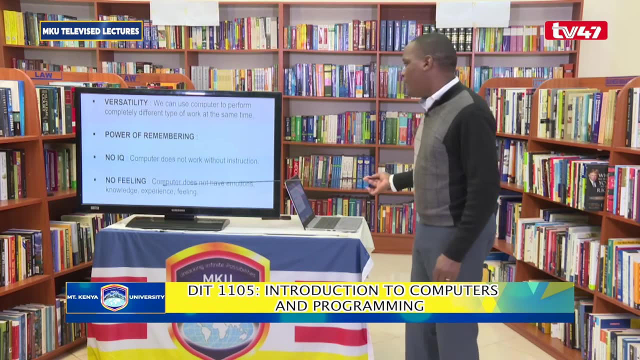 Therefore, whatever you instruct them, they will do that particular task without getting tired, Like the way the human being can work for a long number of hours, They get tired And at the same time enter the correct command. and therefore they they do not have- uh, they do not have- intelligence of. 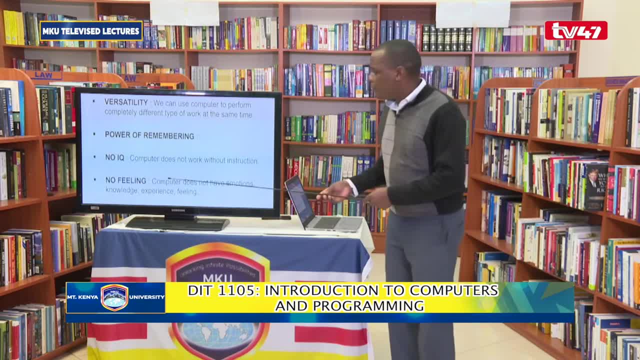 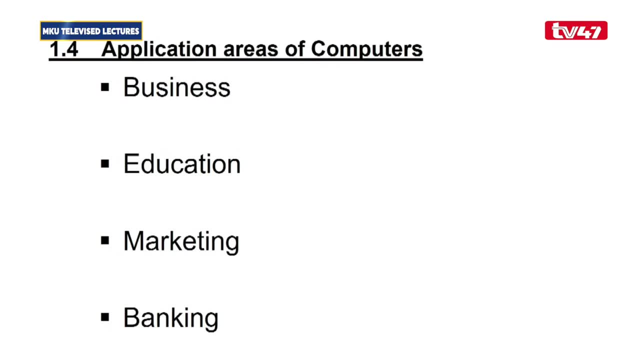 their own. at the same time, they can work for quite a number of hours, especially within a short period of time. the next session is on the application areas. we have quite a number of application areas where we can use the computers. basically all areas of our day-to-day life you can use them. 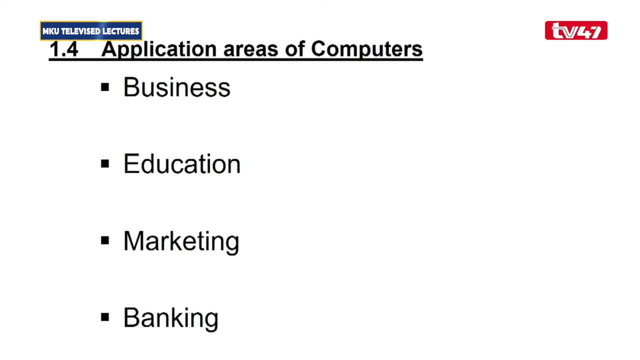 in business. you can use them in education. you can use them in marketing, in banking or the task that requires the application of computers, then they are the most appropriate in business. you can use them for online shopping. you can use them for marketing products. in education, you can use them for accessing a online education. 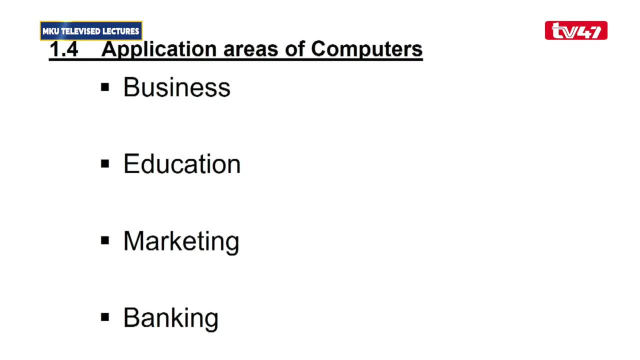 or materials, researching materials. you can use them for taking up a course, especially through distance learning and so on. on the marketing aspect, you can use them for marketing product through the social media platforms. you can use them to market product through digital marketing aspect. you can do banking through the computers, especially through 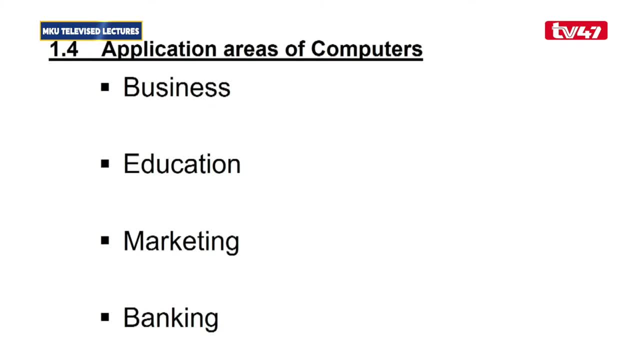 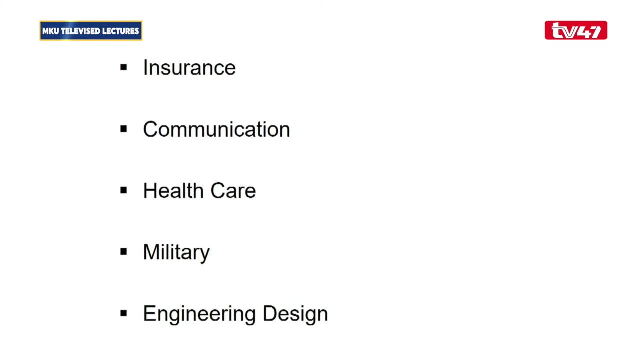 online, online banking and quite a number of areas, especially in our day-to-day life. we also have insurance aspect. we also have the communication application area, the healthcare, the military and the engineering design, where each one of these sections touches our day-to-day aspect of human life. in communication, mostly we use them, especially in sending an email, we use a. 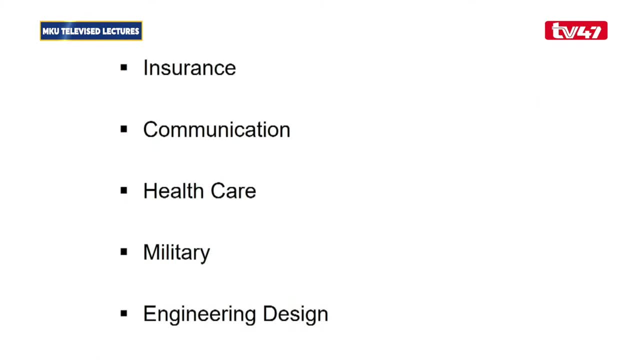 computer. when you are chatting through the social networks, you can you also use the computer. the patient data can also be stored using the computer, and the same can be tabulated and manipulated through the use of computers in manufacture of uh weapons. mostly in the military aspect, we use them. 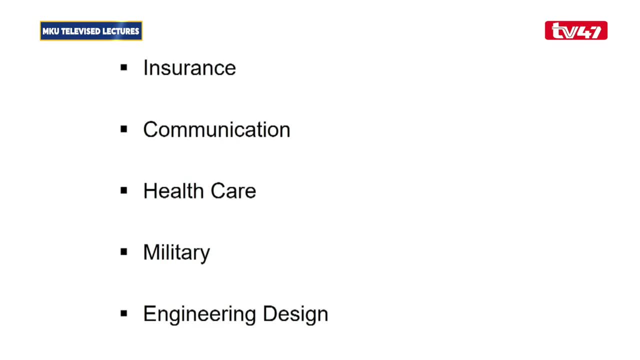 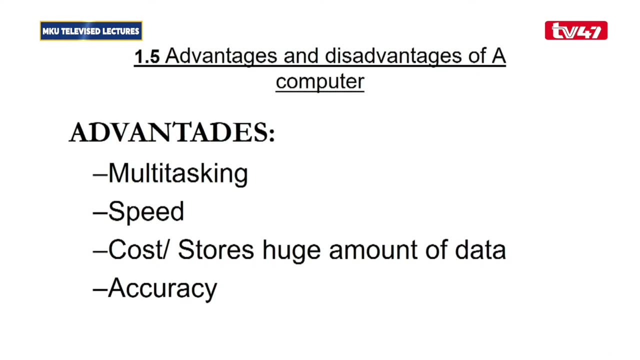 for that particular aspect. so almost each and every area of a human life uses computers directly, and these computers have quite a number of advantages and disadvantages, and the main one is the use of the ability to perform multiple tasks at the same time. they are multitasking, they can do one or more tasks at the same time, unlike the other. 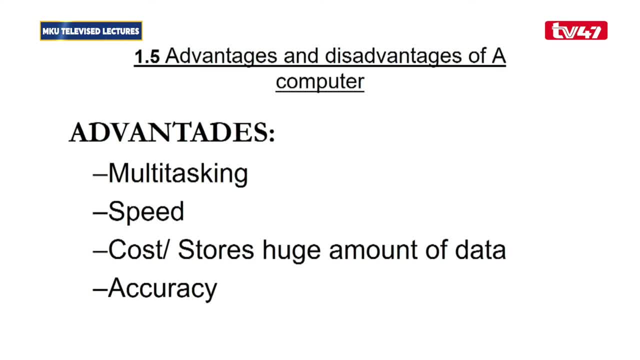 purposes. they can do multiple these tasks at the same does more multitasking. they can do one or more tasks at the same time. unlike the other difficulties you can see, the amount people do is minus twenty-two percent Covid for many cases. unlike the human being, people can perform that with the speed and again. 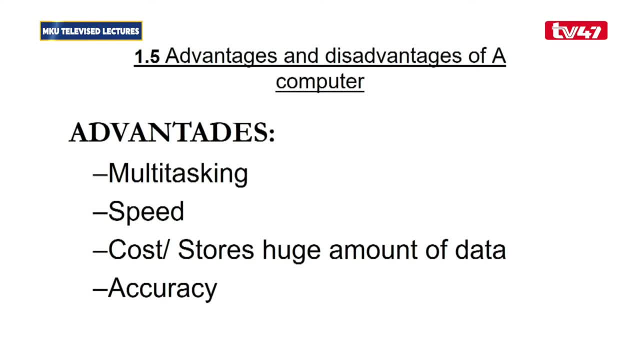 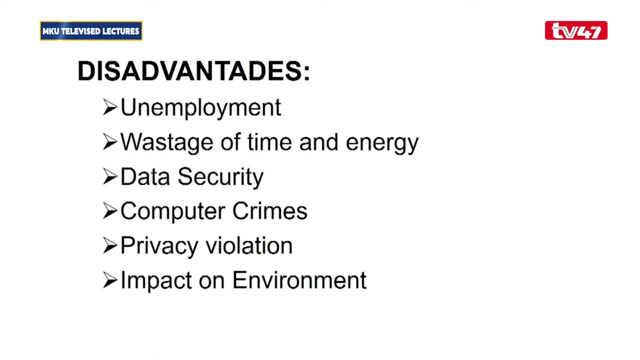 they are cost efficient in terms of cost and the storage of huge amount of data that would require to be stored on large spaces. that they are best at. that. they are accurate in terms of the output also. they also have a disadvantage in that the cost is unemployment, because some of the tasks that a human being would do 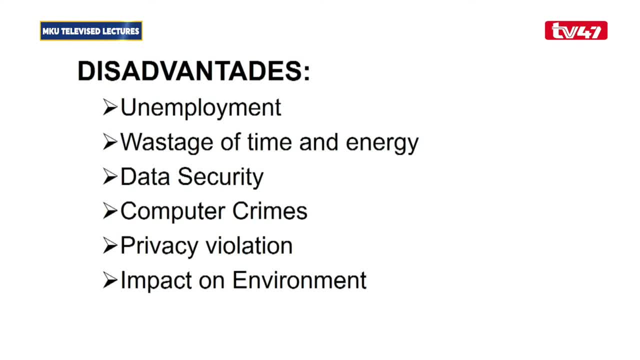 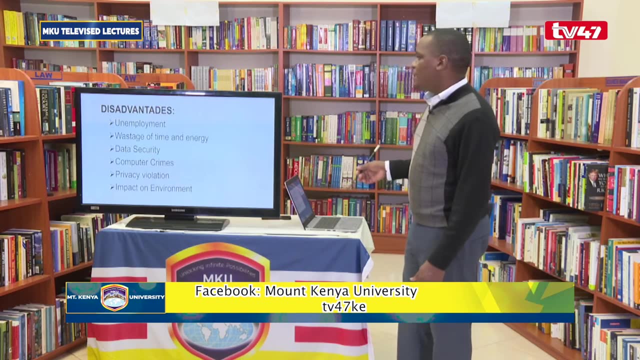 individually, or people would be employed to perform certain tasks, then the same can be done by computers. maybe tasks that was done by two or three people can be done by a single user using a single computer and therefore the cause: unemployment again, sometimes because they are addictive, because a lot of 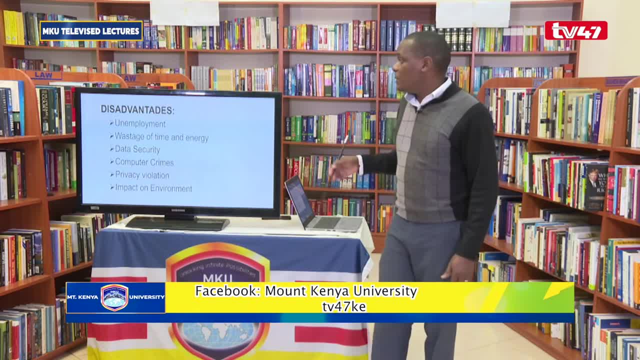 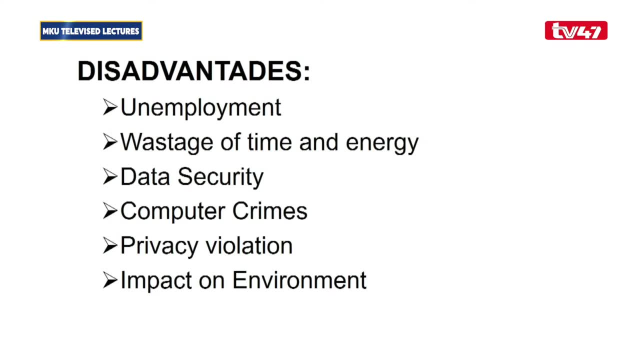 wastage of time and energy. especially when users become addicted to social media networks or in gaming, then they spend a lot of time on games and social media and therefore head up wasting a lot of time because data security- especially sometimes when we have hackers getting into personal information, it one can lose the 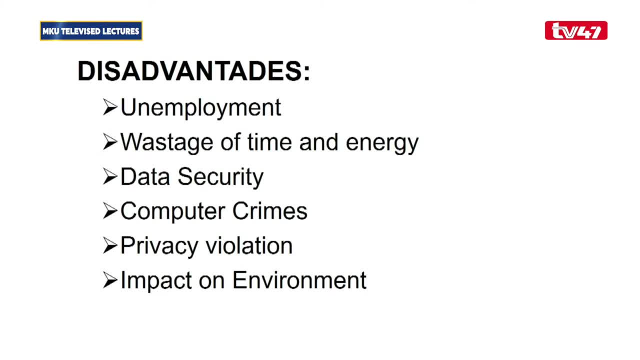 information. as a result of the aspect of data security, computers have also been used to perpetrate computer crimes or resort to crime, where people or the people can steal data from other users, such that information that is made to be private is available or available to the unauthorized users, and therefore resulting to privacy violation of people's data. as the 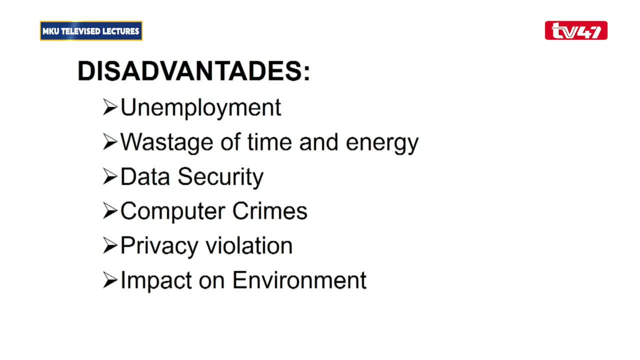 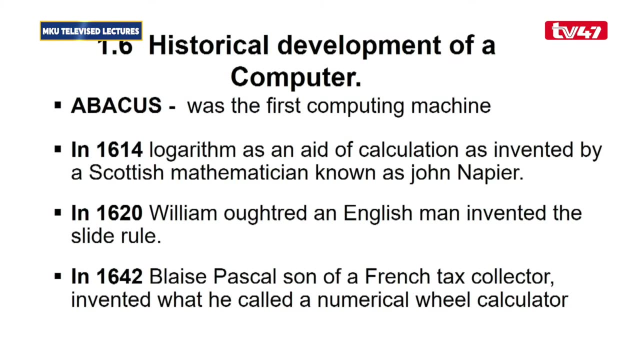 same time, they also have an impact on the environment, where computer parts that are disposed of can cause a health hazard to users if they are not well disposed. these computers are designed over a period of time, and here we are going to look at the historical development of these computers. what were 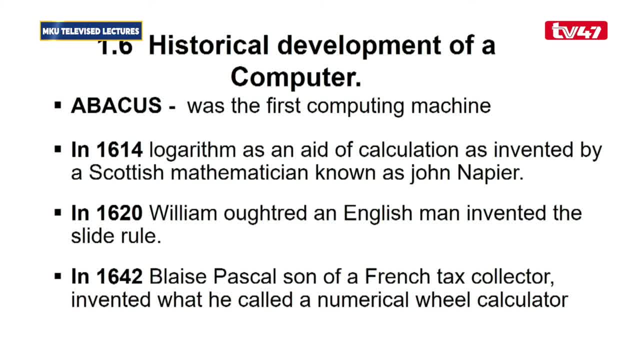 the key electronic elements that were discovered at a particular point of time that were used in the development of these computers, and what were the key electronic elements that were discovered at a particular point of time that, up to currently, what we have as a computer- computer did not start as a full. 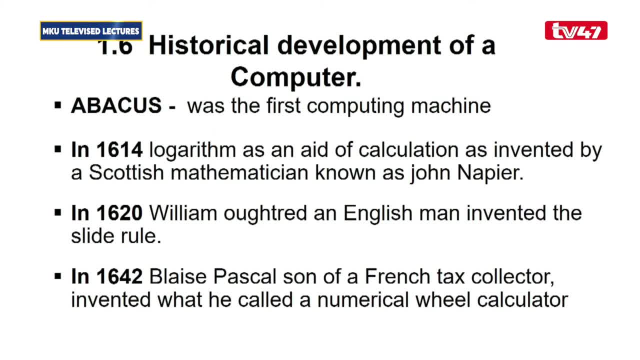 complete computer like we have today. they started somewhere and at each and every time in period, key electronic components were discovered and with continuous research this has resulted to what we have currently as the modern computer. so the first computing device was referred to as abacus, which was which was produced many years before BC, that is, before Christ, and 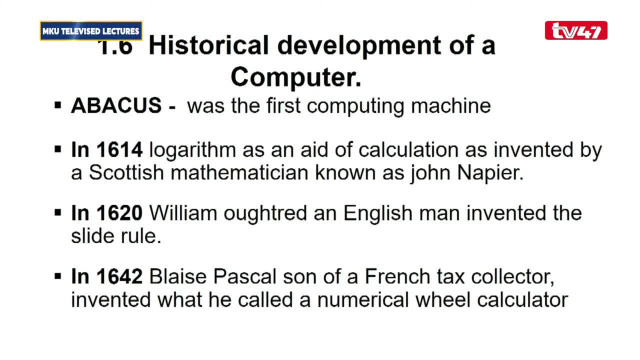 this is dated at around 3000 BC. this computing device. it was a traditional calculating machine or aid that was used by business people of this particular time, 3000 BC- just to keep up with transactions- addition and subtraction- especially with business people. this is the beginning point of the current computer that we have. it is started at this point. 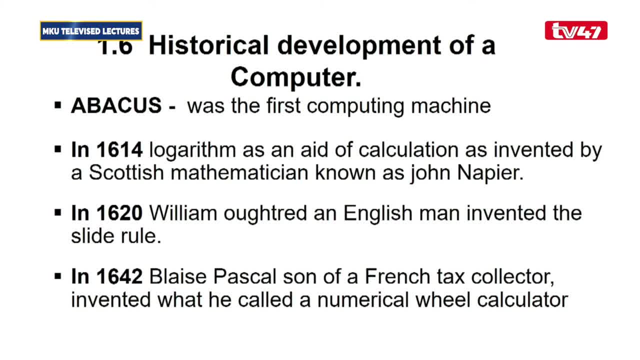 and after this particular device, other key elements or devices were produced by mathematicians and philosophers of this particular, each particular period that contributed to what we have currently and after these abacus. then, in 1614, logarithm was invented by a Scottish mathematician referred to as てον grappier, and this was also another mathematical element of. 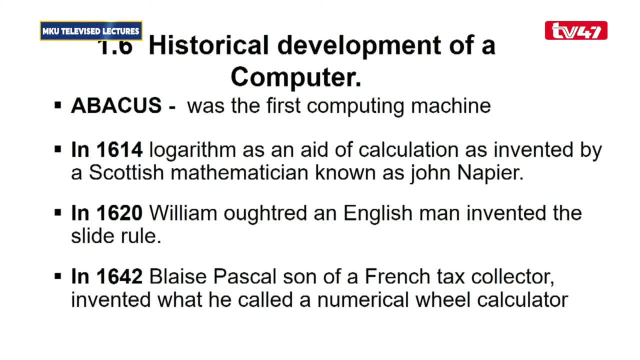 mathematical calculation device that was also used especially in calculation, and later William Ortrid, English man, also invented a side rule and side rule and the logarithm. they are also part of what we have currently as computers, because basically computers were designed as a resort of my mother. 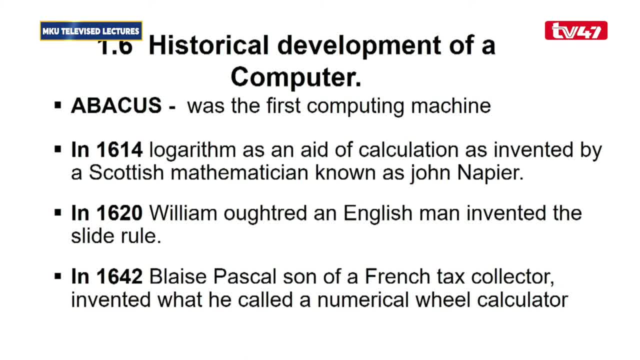 mathematical aspect, the calculation. That's why they are able to manipulate data in a mathematical model. They are based on zeros and ones, the binary digits, and therefore, if you look at the trade, basically majority of the inventors of the key element were mathematicians and philosophers of particular period of time. 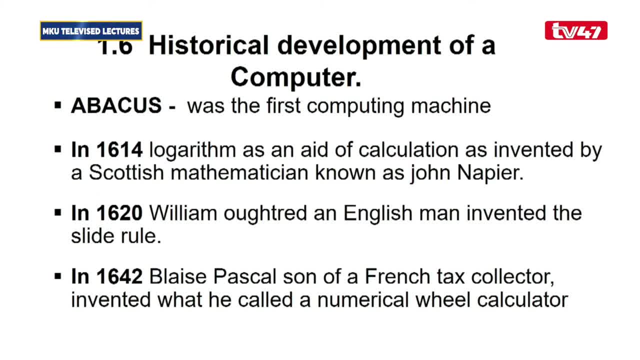 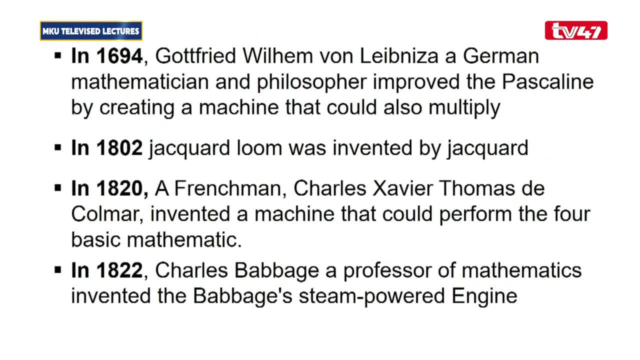 Brace Pascal in 1642, also invented a numerical wheel calculator. Again, this one was to help in the calculation. After this particular time, then, another mathematician and a philosopher came up, improved the Pascal line and created a machine that could also multiply. The other one was for addition and subtraction. 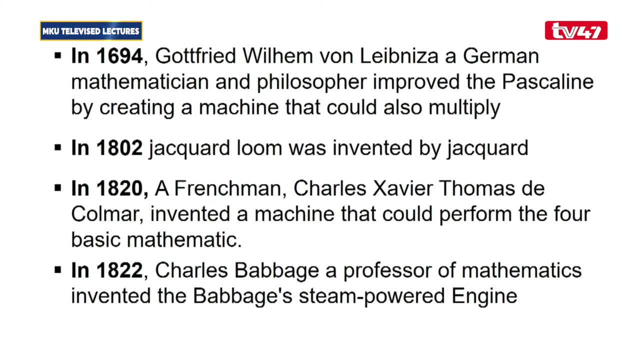 Gottfried Wilhelm also came up with a device that could also multiply, And then later Jacquard came up with the Jacquard Room. This one was also another key invention in the design of computers, because this device was storing instruction in a punched card. 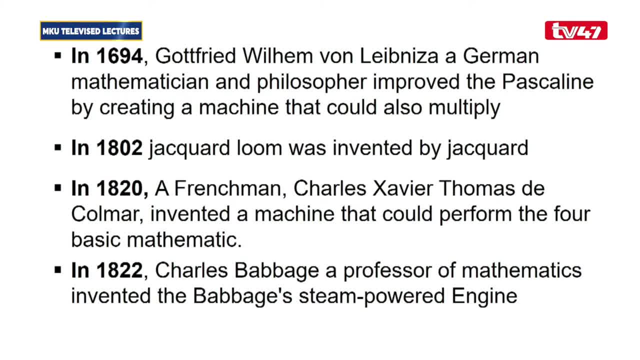 This was an input device that was storing instructions for, to help the people who are carrying out this kind of business, weaving of this particular period of time to store instructions. And then later in 1820, Charles Xavier also came up with a machine that could perform the four basic mathematical functions. 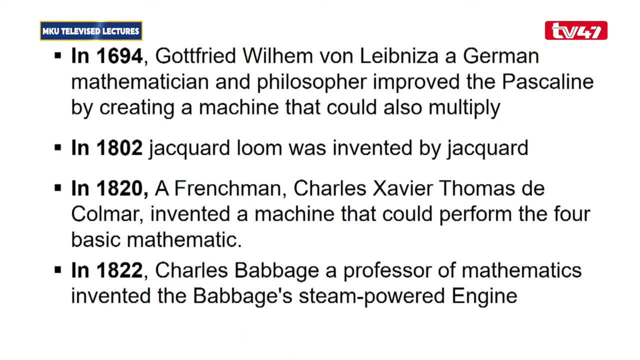 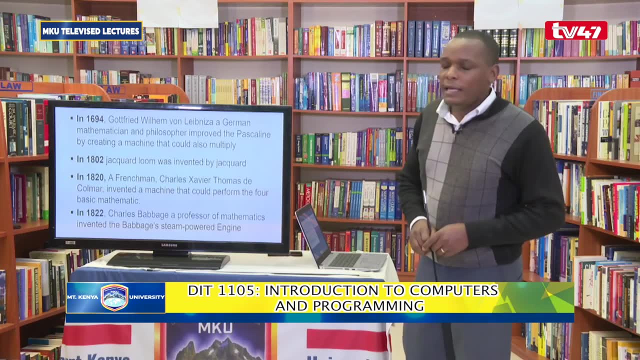 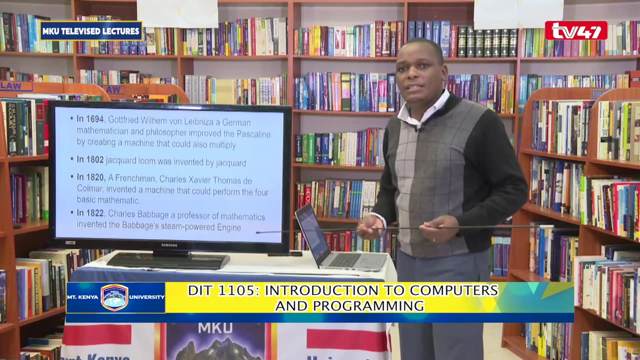 Meaning that it could add, subtract, multiply and divide Again. this was also another calculation device. Then, later in 1822, Charles Burbage, with a Professor of mathematics, also came up with a steam powered engine and later analytical engine Improved it into analytical engine. This is a person who came up with a device that is close to what we have. 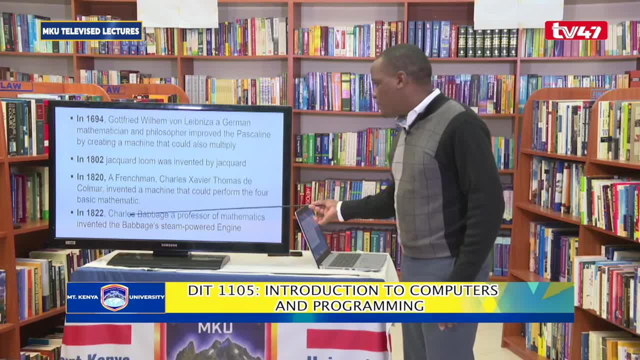 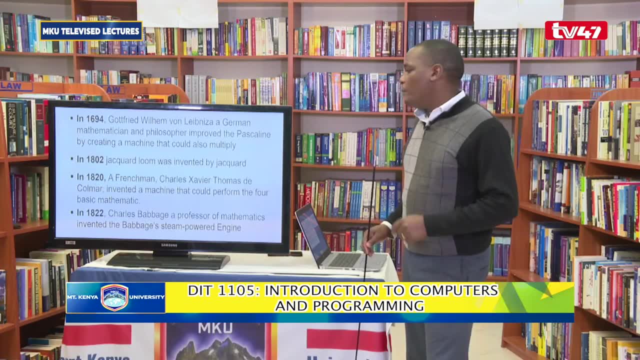 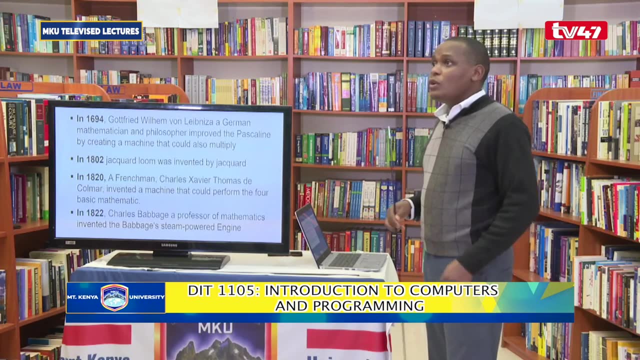 today as a computer, because this device that was produced by Charles Babbage had the four key elements of a computer: It could take an input, it could process, it could store and it could also process. it could also produce an output. 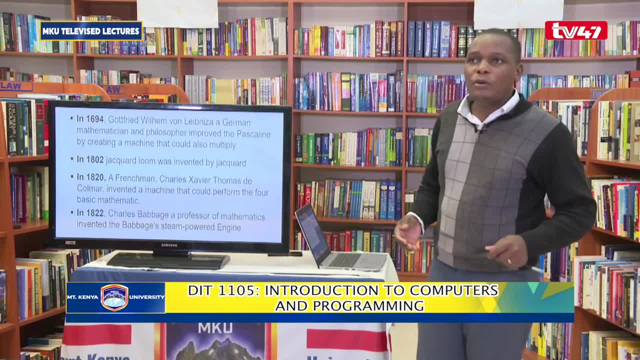 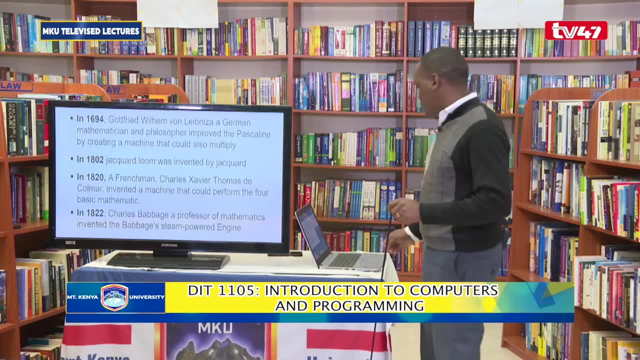 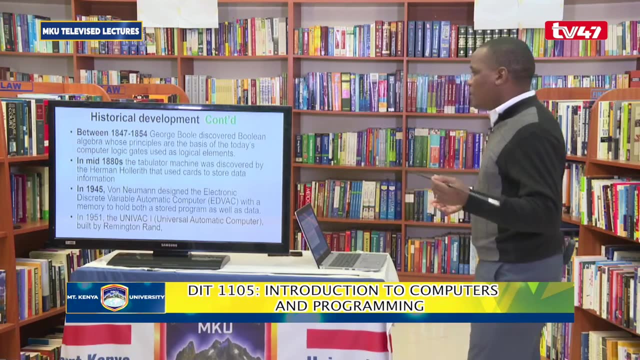 and it could also store. So input, processing, output and storage are the key areas of a computer, which were invented by Charles Babbage, And he's regarded as the father of computers, because what he produced is what the current manufacturers of computers are built on. 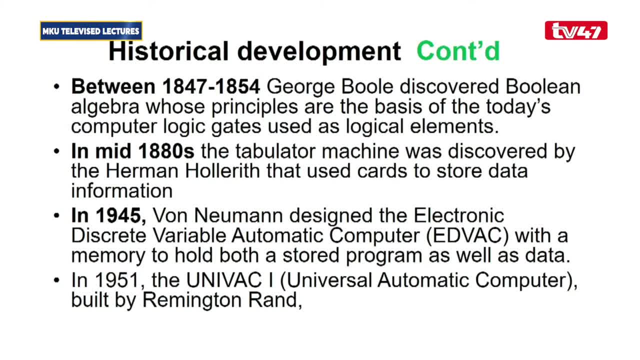 due to the fact that it could perform the key areas, And the same machine that he produced could also be driven through the use of a program. Ridi Adda came up with programs that could manipulate that machine and therefore he's regarded as 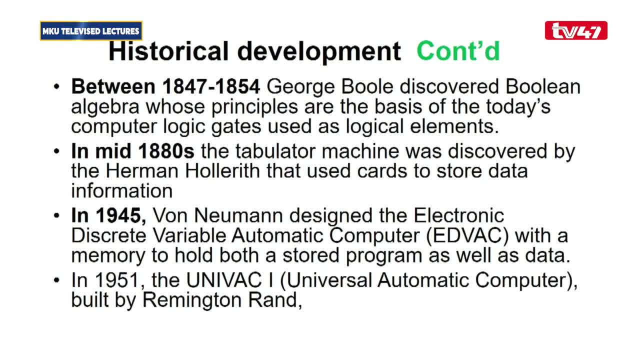 as the father of computers, and what came after it is just improvement of that, especially by George Boole, who came up with the Boolean algebra. And this aspect of the Boolean algebra is used even in today's computer logic gates, which are used as logical elements, and they are implemented in modern computers. 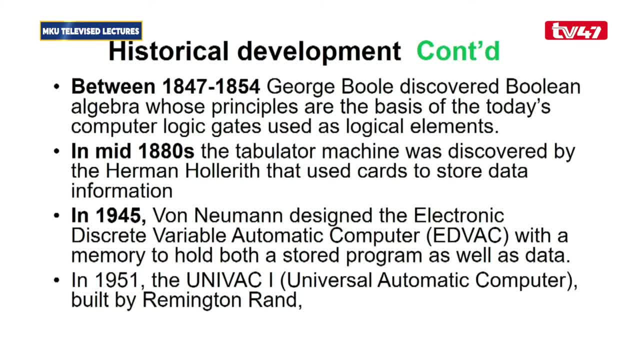 In this particular time, 1880s, a tabulator machine was also discovered by Herman Holley, who used a card, in this case a purged card, to store information, And these were used as input devices that were discovered by Herman. 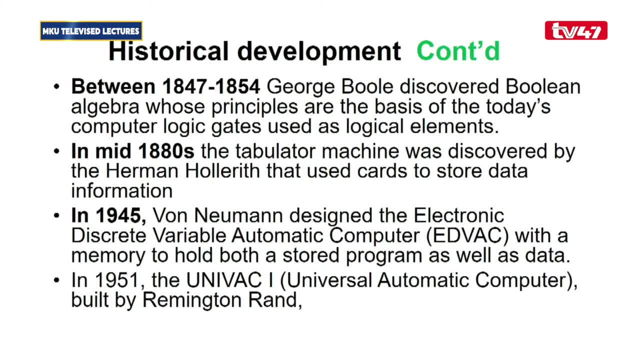 And then Von Neumann designed a discrete variable automatic computer. That was around 1945. And later, in 1951, a universal automatic computer was built by Remington Rudd. And these again were built on the previous discoveries, actually from Charles Babbage. 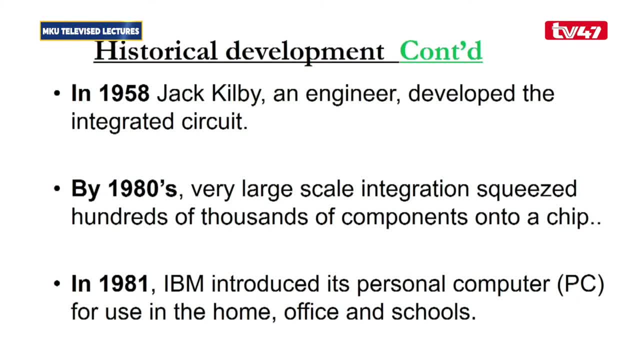 And what resulted was a much, much better device. Later, in 1958,, Jakilbe came up with integrated circuits And therefore what resulted is a more integration of components, resulting into a smaller device, which is now. the computer size became smaller and smaller. 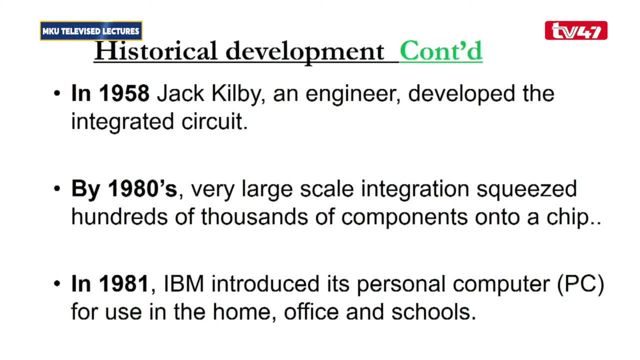 as the key electronic elements came about. Remember, initially we started with vacuum tubes, then later went to integrated circuits or IC, resulting into a much smaller computer And, with the time, until now, the ability to squeeze more components into a small circuit board. 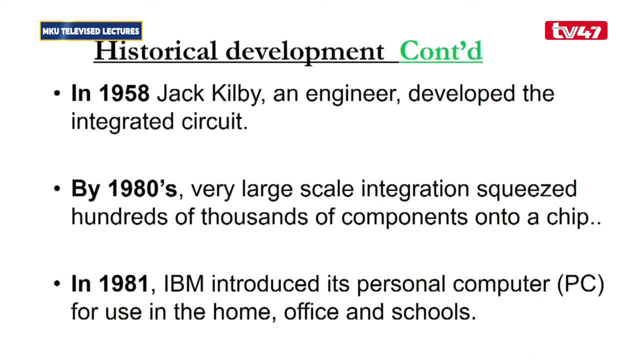 a small silicon board is the process that is taking place, And after integrated circuits we went to large-scale integration, resulting into a smaller computer and very large-scale integration. And by the time we go, By 1981, IBM introduced the first personal computer that could be used in homes, office and in schools. 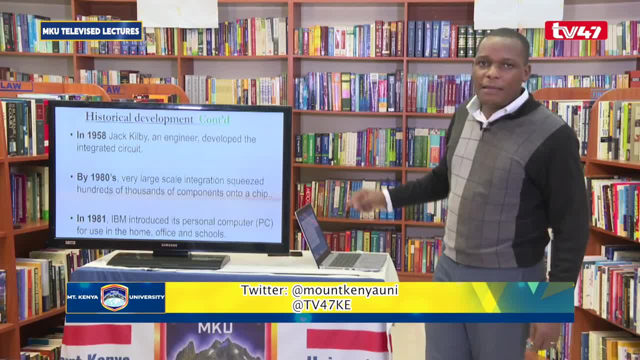 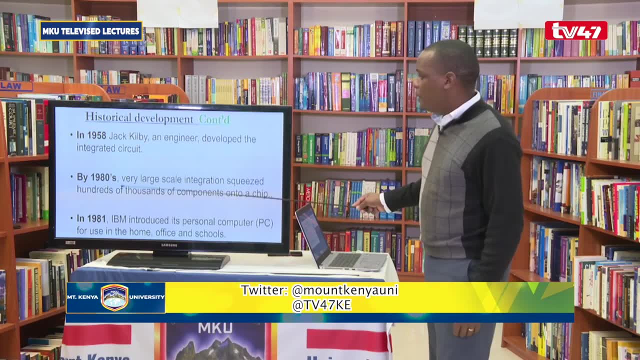 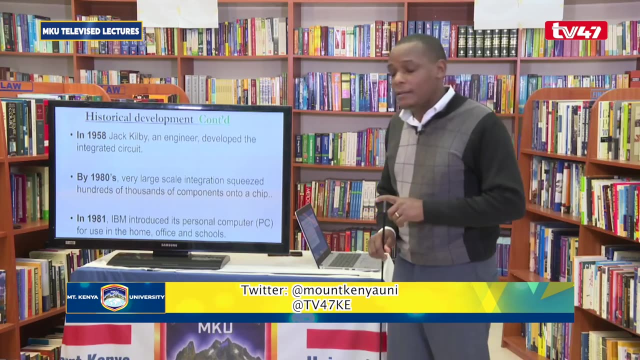 So these computers started somewhere a long time ago, with key discoveries of individual components and, with the time, improvement of each and every component resulted to what we have today as a personal computer or a PC which can be used by individuals. 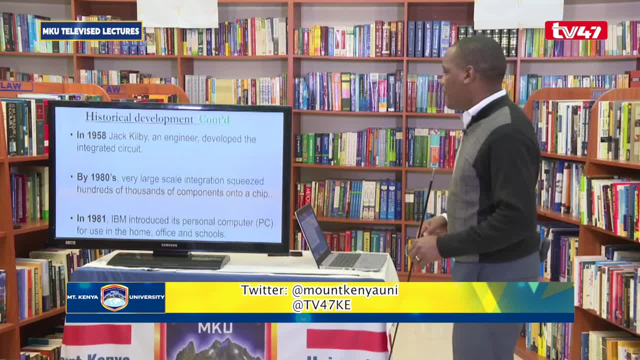 either at home in the office, in the classroom or in the classroom, either at home in the classroom or in the classroom, or in the classroom or in the classroom, and so on, And as time goes on, even currently, computers are becoming smaller in size. 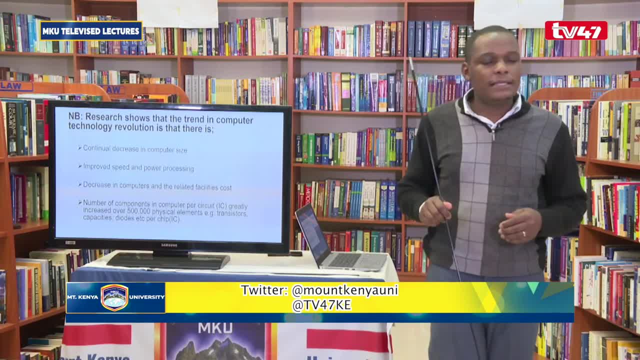 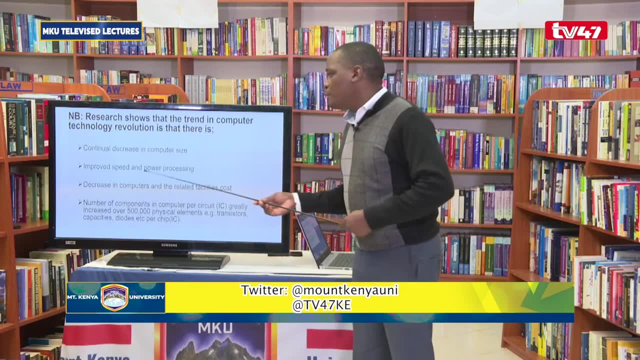 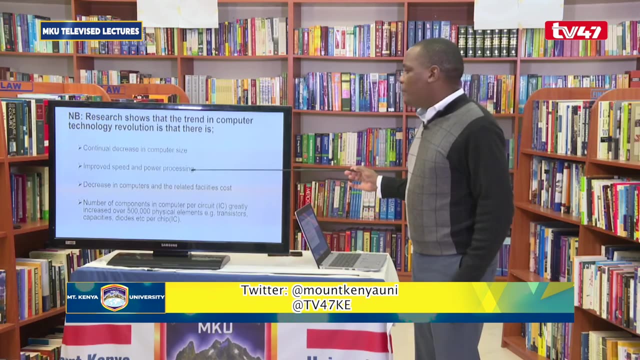 due to that ability to integrate more components into a small circuit board, referred to as integrated circuit. The power of computers in terms of speed is also increasing. As the days go on and key discoveries are being done. the processing speed of computers is improving and increasing. 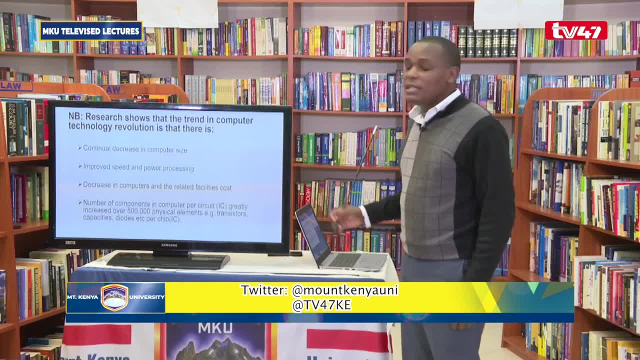 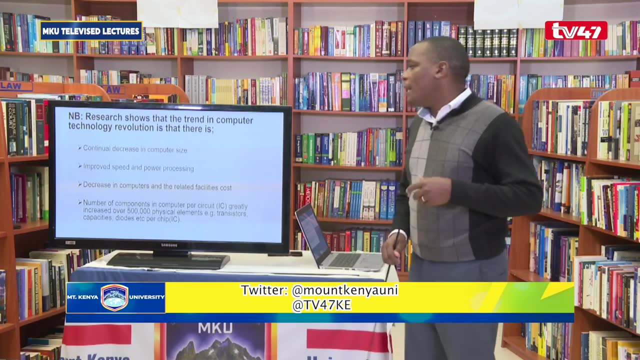 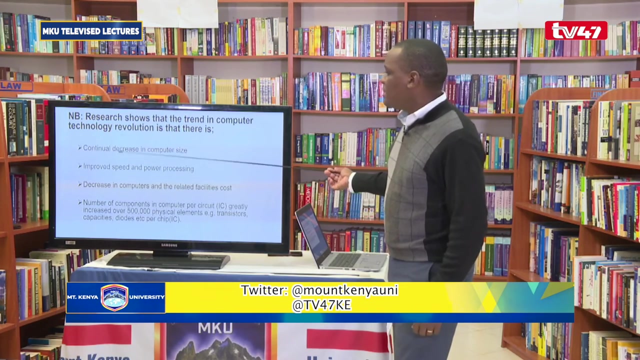 And then their prices are also reducing due to new and better discoveries and improvement, and as more users even acquire those computers, then their prices are going down And with that then more people are acquiring those computers and by 1990s- that is when, due to massive acquisition of computers, 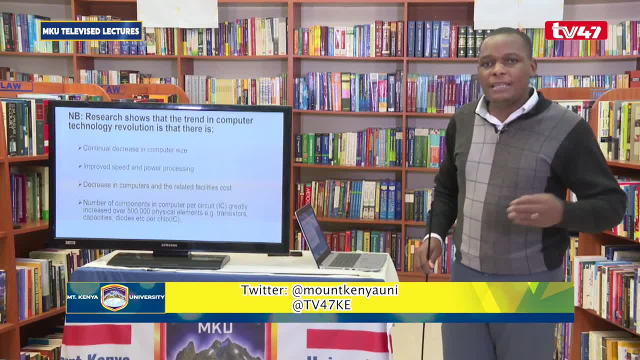 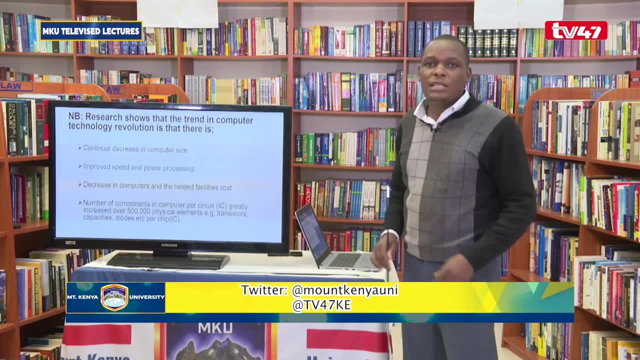 that is when they need to connect them together So that different users can share resources came about, And that was the technology. the networking technology came about And through that interconnection of computers together has led to what we refer to as the global village. 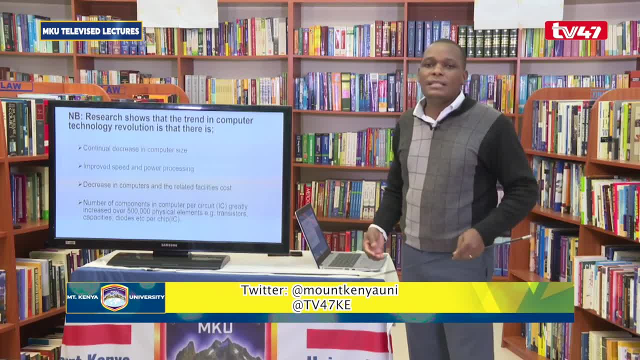 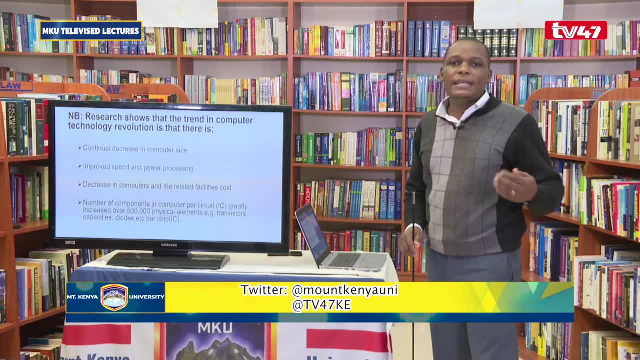 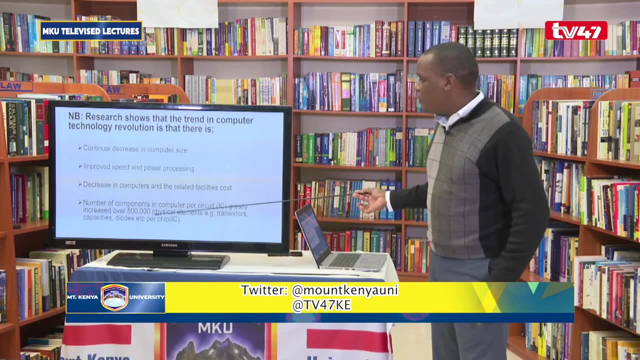 because you can communicate with different users within the entire group, Like you are within a small village Today, you can send an email and the recipient might be miles and miles away from where you are. So you communicate like you are within a small area. 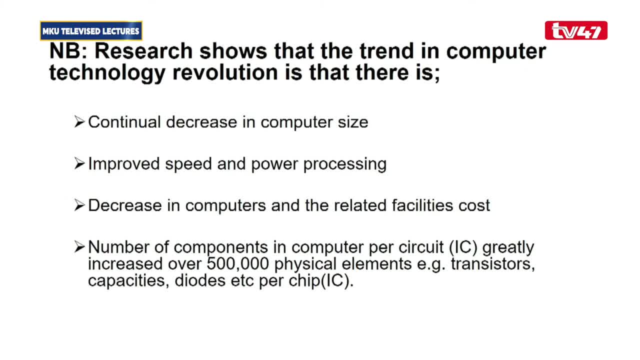 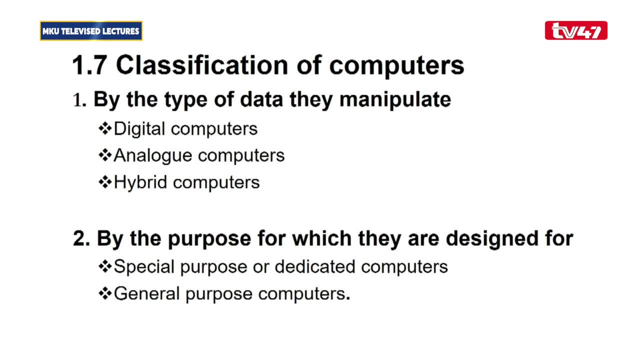 due to the fact of that, these computers can be integrated together, connected together, such that they can communicate in a network. So that is the historical development of computers and which has led to what we have today. All those computers can be classified based on a number of categories. 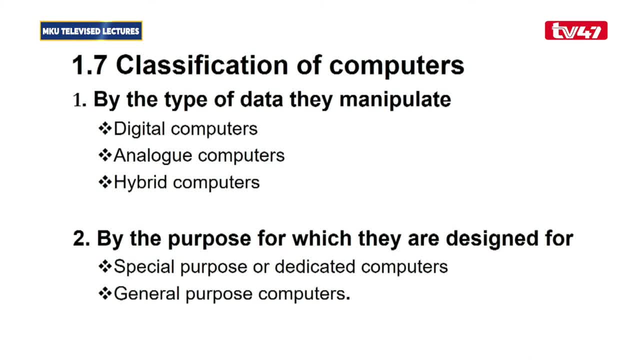 We call them by the type of data they manipulate. There are those computers that manipulate digital data, and therefore they are digital computers. There are those that manipulate analog data, and we also have a hybrid, a mix of both digital and analog. 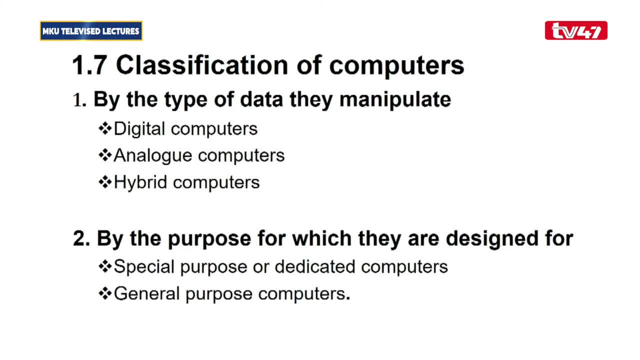 Digital computers. they manipulate data in form of zeros and ones, the binary data, And this data is a discrete variable, Not a continuous, And these are the most common computers that we have within the group. They are digital computers, But there are those that measure variables that are in continuous form. 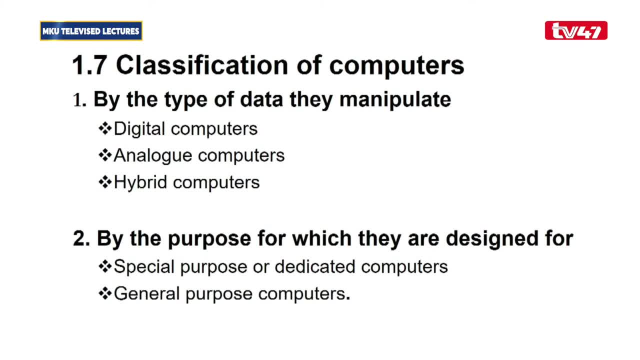 Like the ones that measure variables like pressure, things that are in continuous form. That category of computer is referred to as the analog computer, And there are those that measure both digital and analog. analog: They can measure discrete variables, numbers and at the same time. 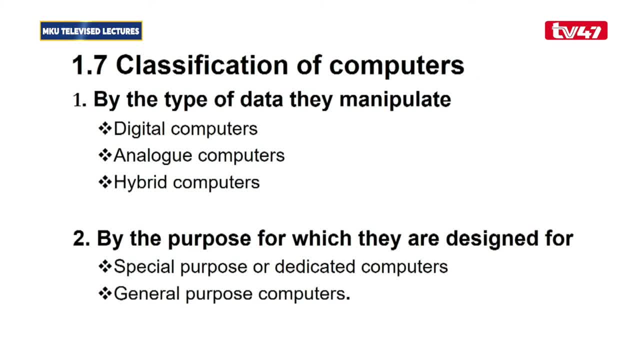 they can measure continuous variables. They are referred to as hybrid computers, like the ones computers we find in an area, like in a petrol station, where that computer is measuring the pressure of the fuel from the fuel tank. At the same time it is calculating the prices of that fuel that is getting. 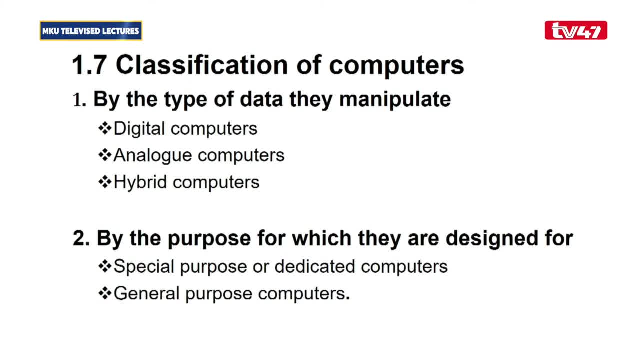 out of the tank in the form of variables, digits, numbers, the price. So you find that it is measuring two variables at the same time and therefore it's a hybrid computer, given that it is dealing with both digital variables and analog values. We also have a classification based on the purpose. 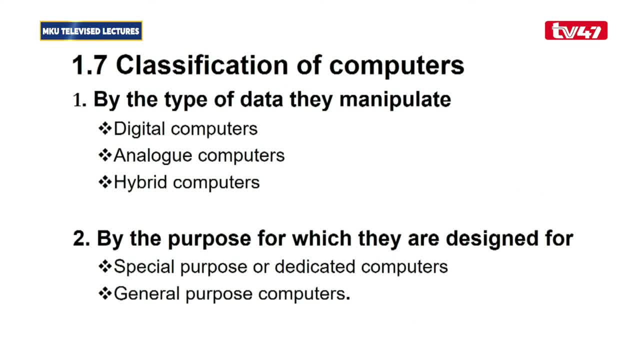 of the fuel. We also have a classification based on the purpose of the fuel. We also have a classification based on the purpose of the fuel. We have special purpose computers and general purpose computers. Special purpose or dedicated computers: they are computers that are designed for a particular purpose. They 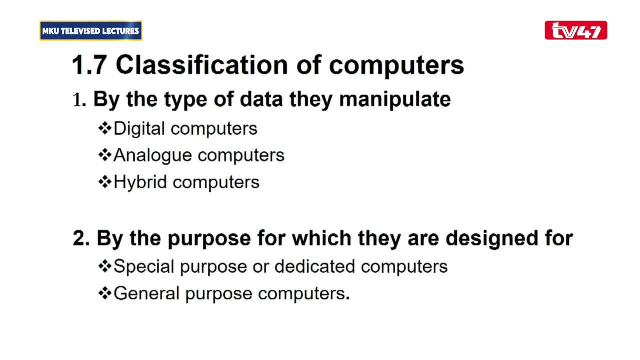 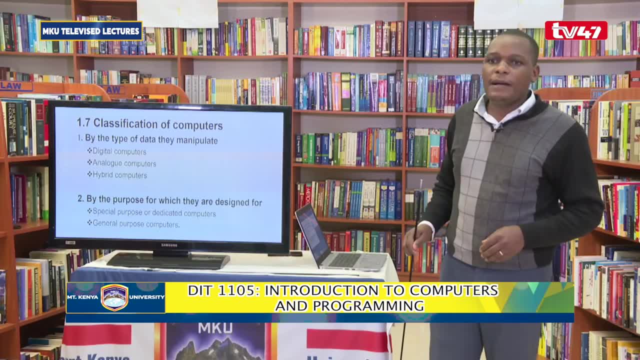 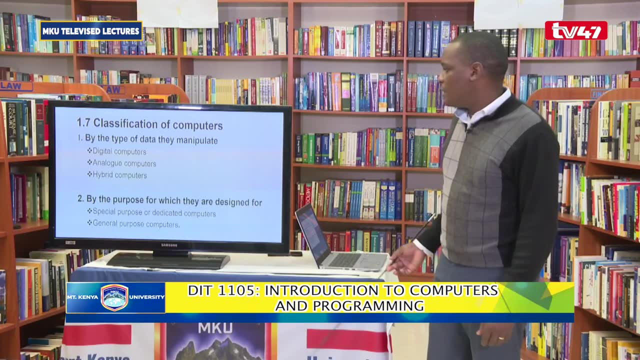 are designed to perform a specific purpose. Let's say you have a computer that is designed for generation of ammunitions in a manufacturing farm. They cannot be used in an office for general use, maybe typing and printing and doing other things. They cannot be used in an office for general use, maybe typing and. 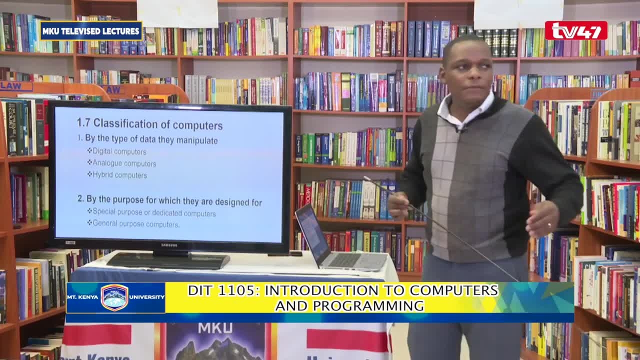 doing other things. They cannot be used in an office for general use, maybe typing and printing and doing other things. They are generally designed to work in a manufacturing farm. They are those that are designed to work in an hospital to monitor the progress of a 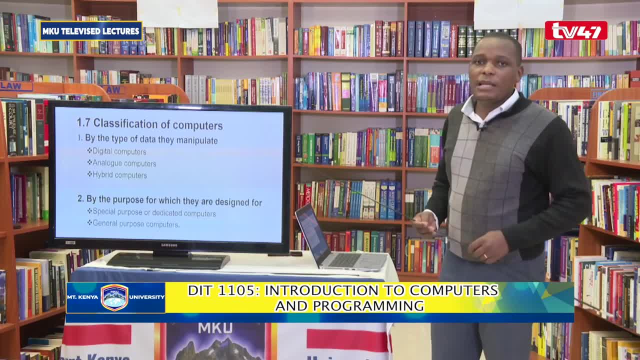 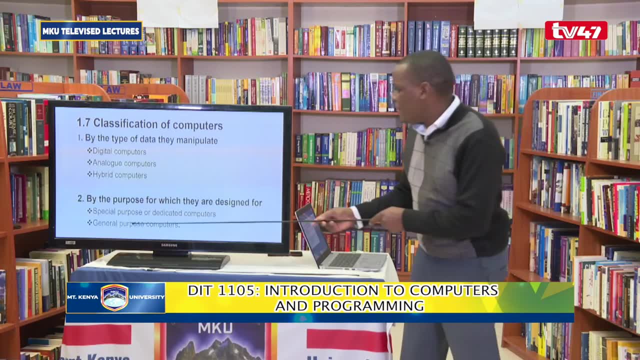 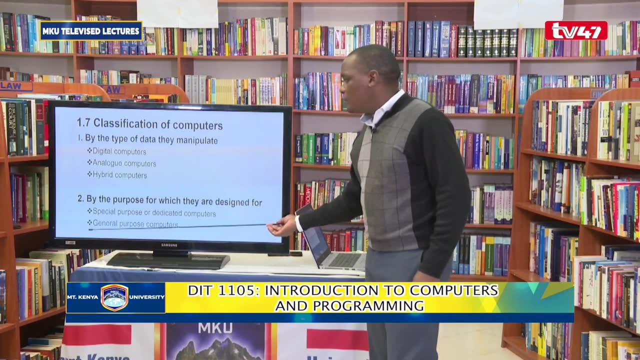 patient. They measure the blood pressure, the sugar levels and so on. Those are special purpose computers. And then we also have general purpose. You can use them for any task, so long as you configure them to that particular task by installing the relevant software. If you want to type, 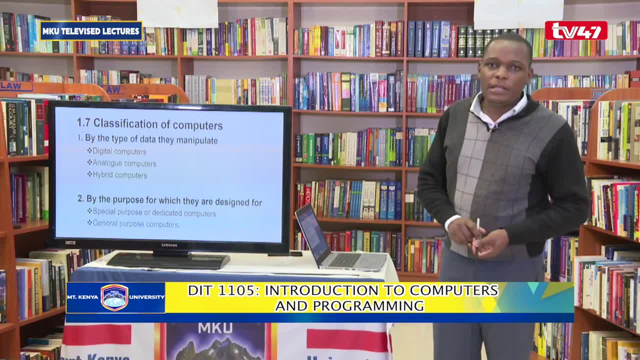 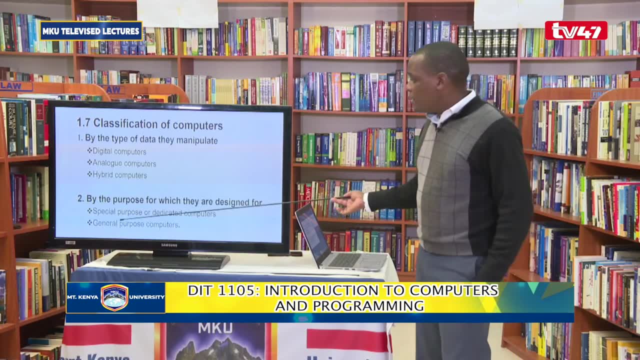 you configure the computer to use an application like Microsoft One. You can use the same computer to carry out computation- mathematical computation- by using the appropriate application program, like spreadsheet. You can use the same to manage the database record by using a database application. You can use 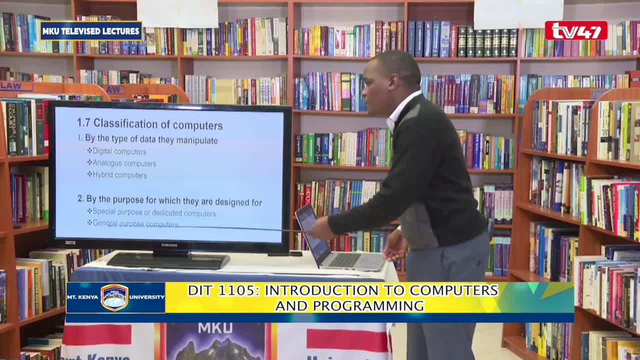 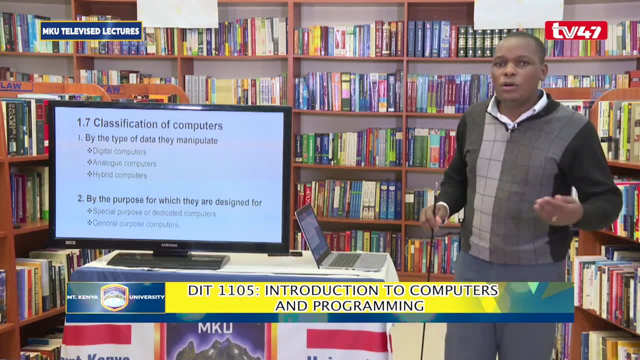 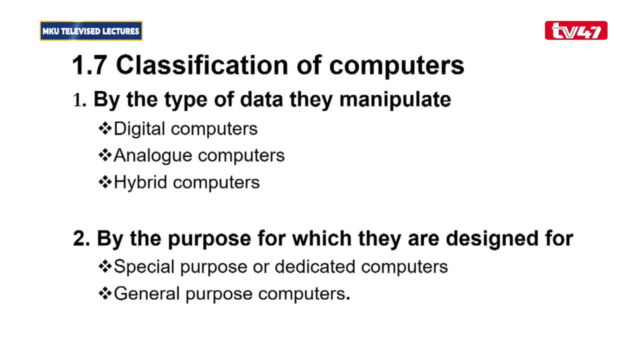 the same computer to make a presentation by using presentation softwares like PowerPoint. So you can use them for general purpose. it depends on what you want to do. if you want to draw, you do use a drawing software. if you want to do a graphic design manipulation, you use graphic softwares. so they are general. 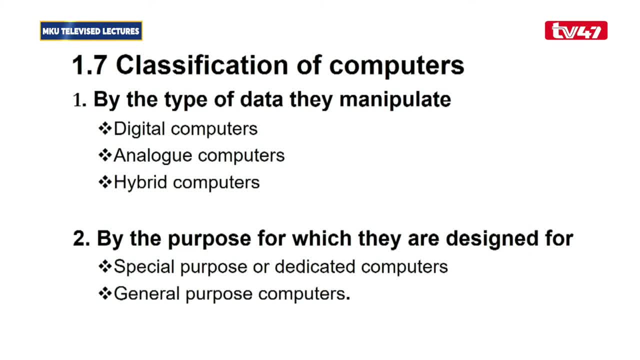 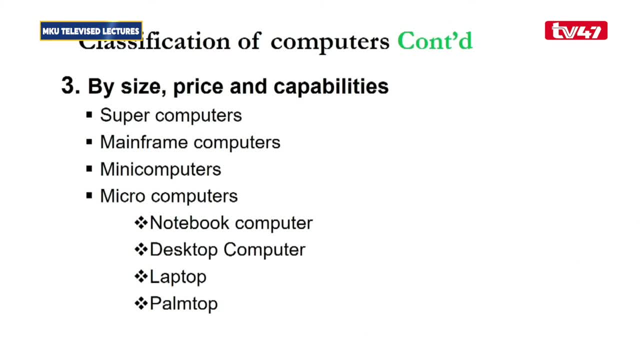 purpose. it depends on what the user wants to perform using those computer. so they are also classified according to purpose. then you can also classify them according to the size, price and capability. this is one classification where under this classification we have supercomputers, main frame computers, mini computers and the microcomputers. the order here is in form of the. 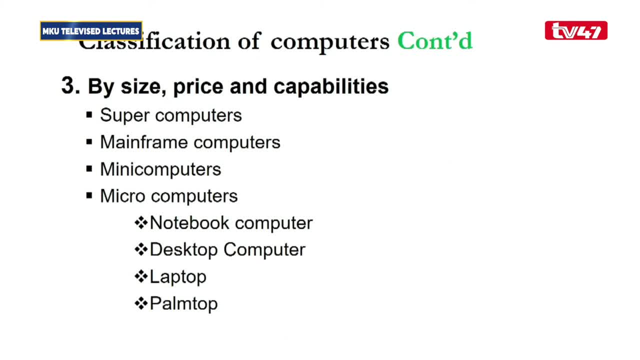 size supercomputers are the largest. mostly these are not used by individuals. they are used to manage records, especially where large, huge computation is required, especially in government sections where we have huge volumes of data is required, or like especially in parastatus or in areas where 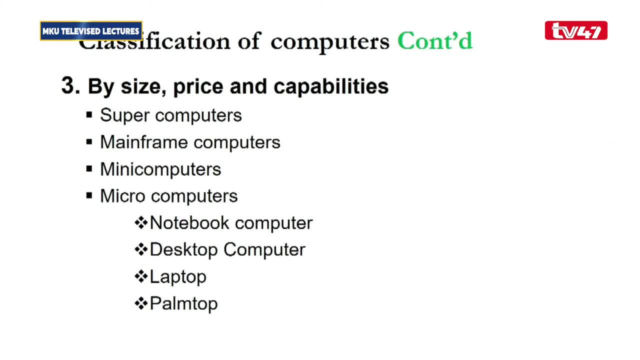 huge competition is involved. this super and mainframe. they are not used as individual computers, they are main. maybe if you look at an area like in the registrar persons, you expect a lot of data in such such a section where you have each and every person within a country, their data. 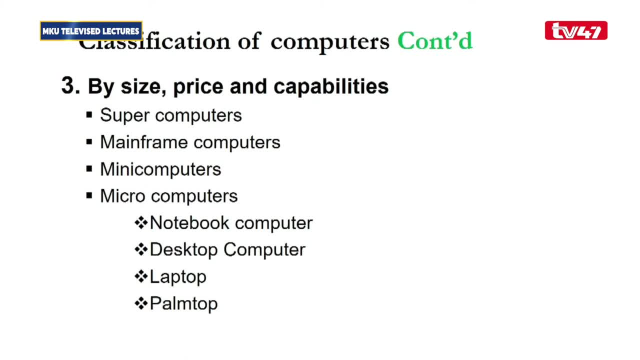 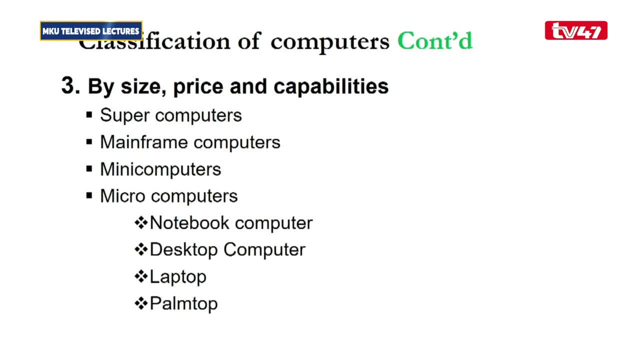 work also in areas where large competition is involved, but not as much as in a supercomputer. so you'll find them again in areas like in companies, uh, medium-sized companies in hospitals. so you'll find them again in areas like in companies, uh, medium-sized companies in hospitals. 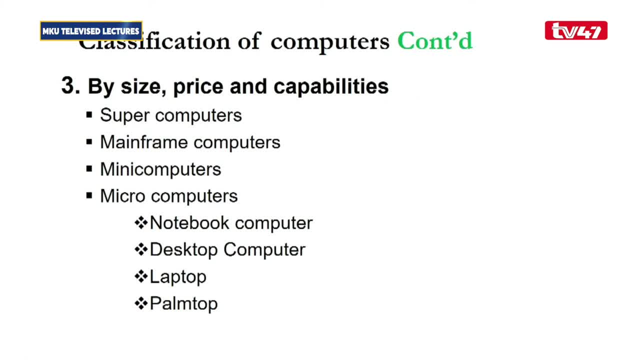 all in sections where a large volume of data is also involved, but not as much as in supercomputer. so they are smaller than supercomputers and then many computers. they are again smaller than super and mainframe computers. they are mostly used as servers. also they are not used as individual computers because, again, they are huge. they. 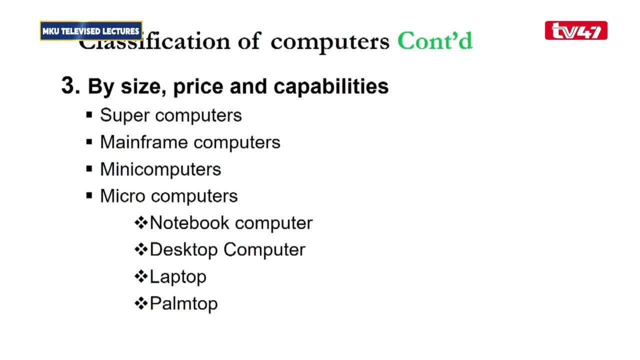 process a lot of data. and then we have micro computer. they are the smallest. micro means small. therefore these ones are used as individual computers or as personal computers. they can be used by individuals and they also vary in size based on the type. we have the notebook. there are small computers which can act as a notebook, where you can put a small point as 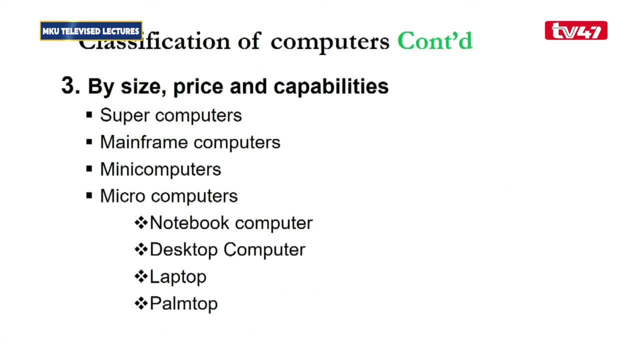 as, like a notebook, we have a desktop computer. this is a computer that you can use while placed on a desktop. as the name indicates, a laptop, you can place it on your laps and the palm top. you can place it on your palm. that is the top of your heart, the palm and. 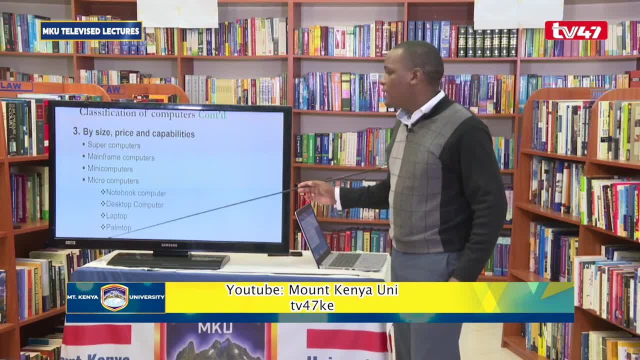 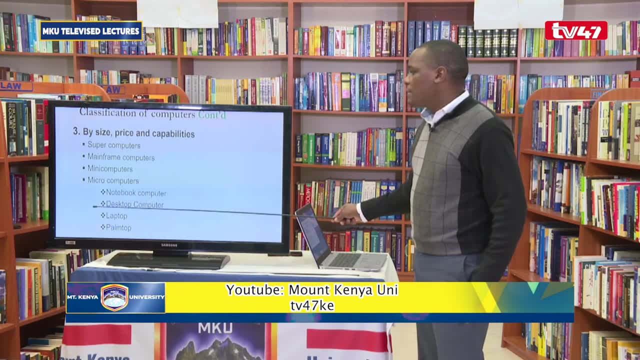 therefore, these varies again in terms of the size and the usage: desktop, the personal computers that you can use as a on a fixed location or where, maybe in an office, in a school. a laptop- it's a portable device, you can move alongside with it and work it anywhere. you can place it on a desk. 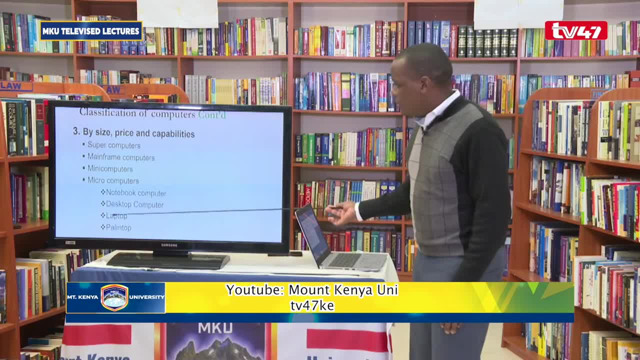 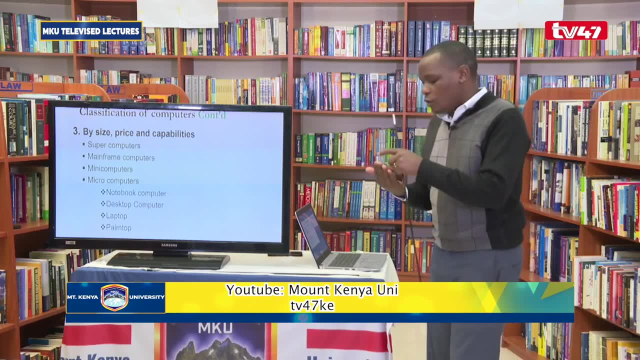 you can sit down and place it on your lap and use it comfortably. the palm top the same. it's a small computer that can place it on top of your palm and use it just like a normal computer. so that's the classification according to the size, the price and capability. and lastly, you can classify them according to generation, where you 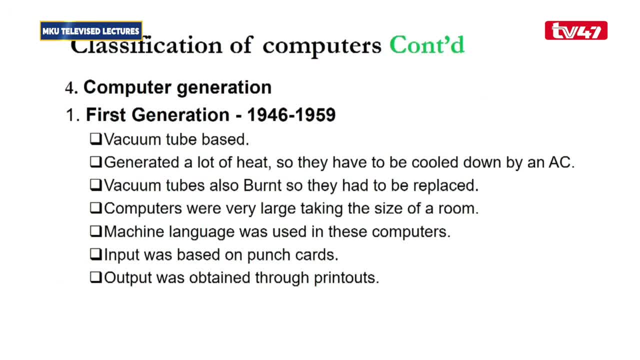 have first generation, second generation, that generation, fourth and the fifth. so each of these classification is based on what we are grouped at, the within the historical developmental computers between 1946 and 59. these are classified as first generation computers, or basically 1940s. these computers are forms, a generation, based on the key element that formed these computers. 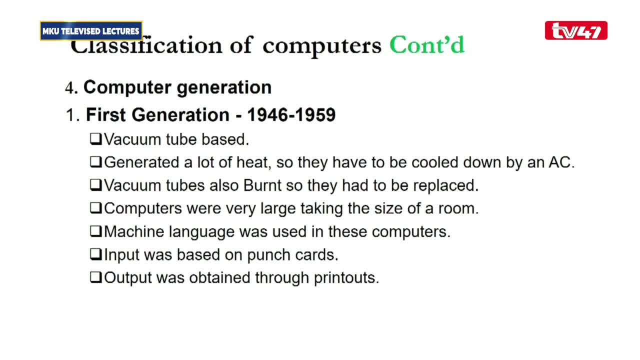 of this time, the first generation computers. the key element was the vacuum tubes. the second generation: the key element were the 결곤 particles, were thehetics of the Gomu a ia, problems about atoms, about radi codings, etc. This group, the lack of Keys and the lack of data, accounts for getting to the Properties and regulations of the Olympics of machine computing, Ops. life of computers involved teaching, infin decisive hp Excel quantities and all that No которой of computers, expenditure of dataخلπ Yoon's were y сегодня eric. this is one of the main, plus one of the most importantagnery. 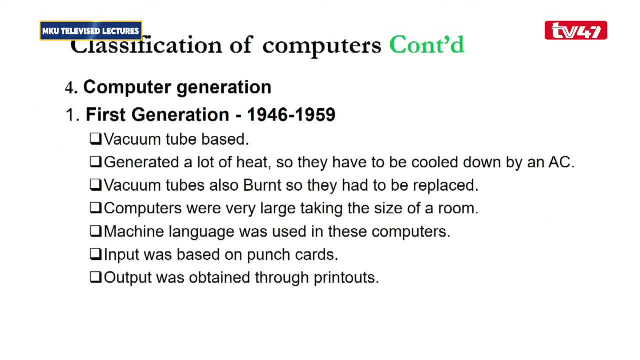 was the. so the first generation: the key element was the vacuum tubes, and these are the computers of 19 1940s. then the second generation: the key element was the transistors, and therefore each of these component forms a particular design and a particular characteristic that result from this. 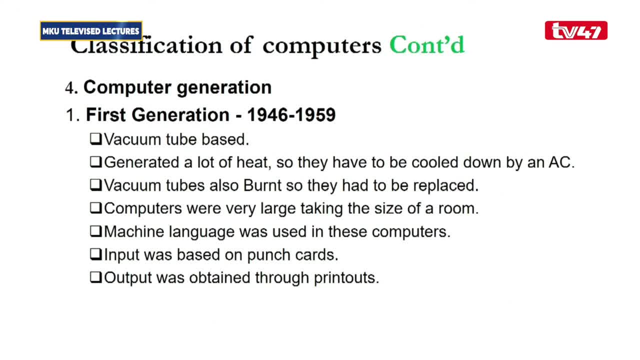 particular computer, like the ones that form, were based on vacuum tubes. they are quite big in size, they generated a lot of heat and therefore they required space, the a single computer could occupy an entire room. they generated a lot of heat, they were very slow and the the input was in. 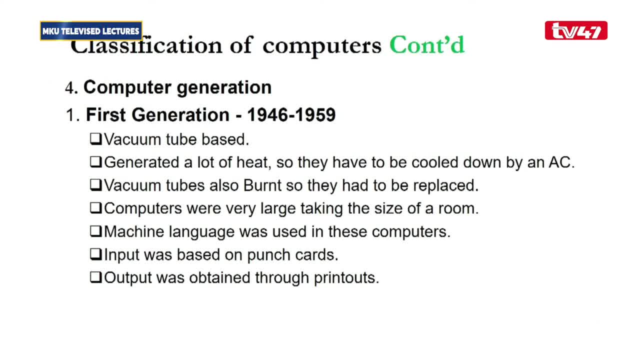 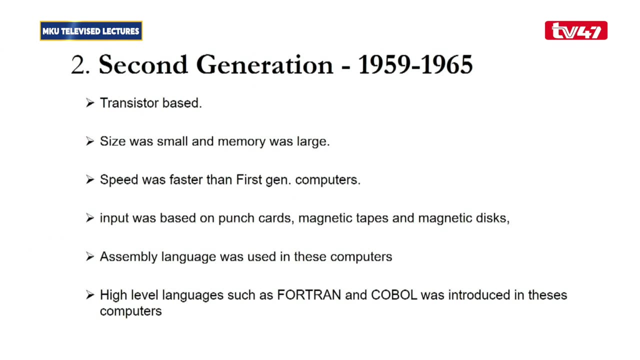 form of punch card and therefore these particular computers were based in this particular period of time. but later the vacuum tubes were replaced with the use of uh transistors and they formed what you call the second generation from 1959 to 65. so the vacuum tubes were replaced with 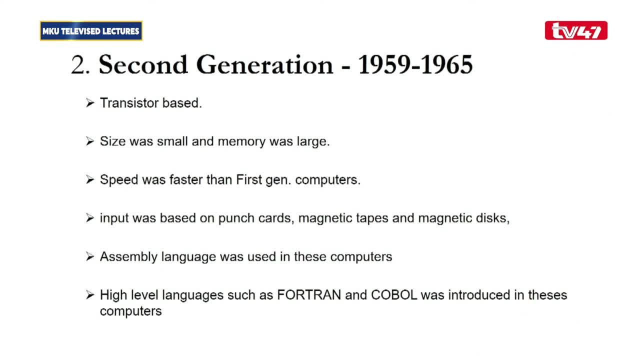 transistors, and what resulted again was a computer with certain characteristics. they were smaller than the first generation, they were faster than the previous generation, they generated heat and then they would be able to perform more in terms of functionality than the previous generation. The input again was also in form of punch card or magnetic tapes and magnetic disks. 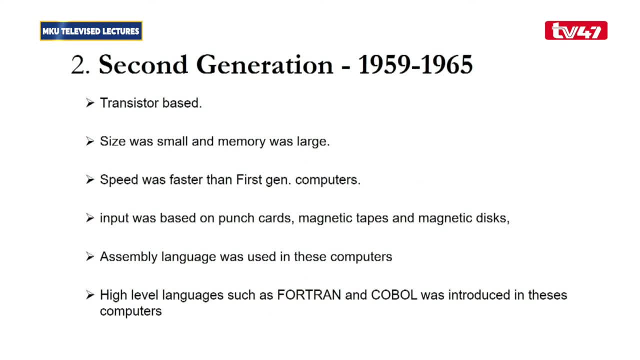 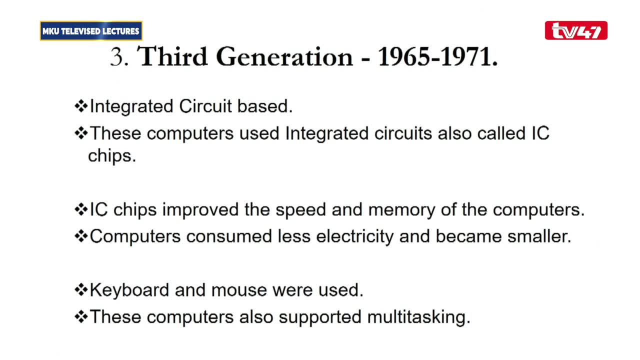 that were used to store data, But later in the third generation, integrated circuits replaced now these transistors and again resulted into another generation, which is referred to as the third generation. So integrated circuit or IC replaced the transistors and again the computer that came. 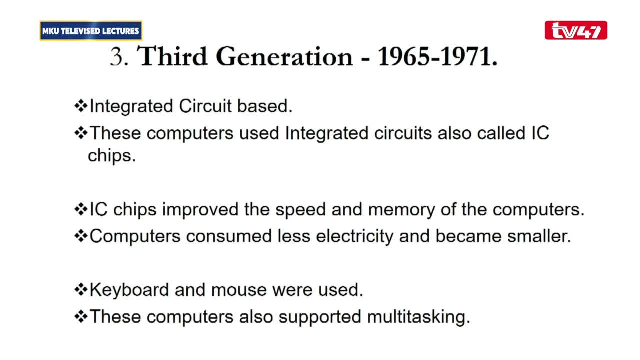 out after that was much better than the first two generations. It was a much smaller computer that was a bit faster, that could store data in a much better way and generated less heat, And after this integrated circuit, the fourth generation resulted into much integration. 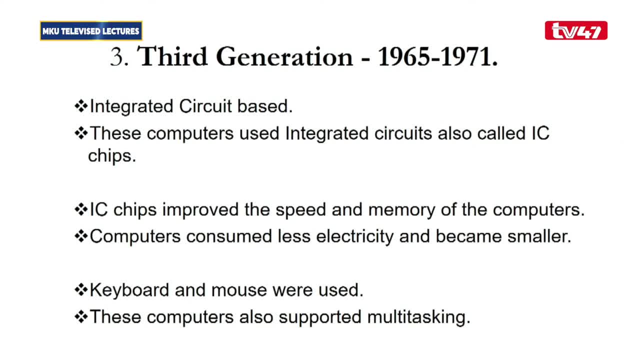 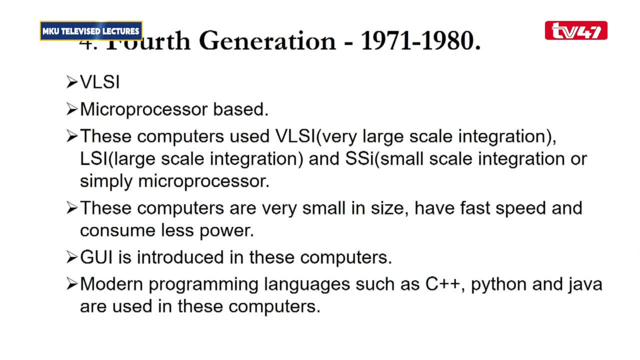 of these components, Which resulted into large-scale integration. The fourth generation was based on large-scale integration, or very large-scale integration, that was based on microprocessors, And this resulted again into a computer that could perform much better than the first three generations. 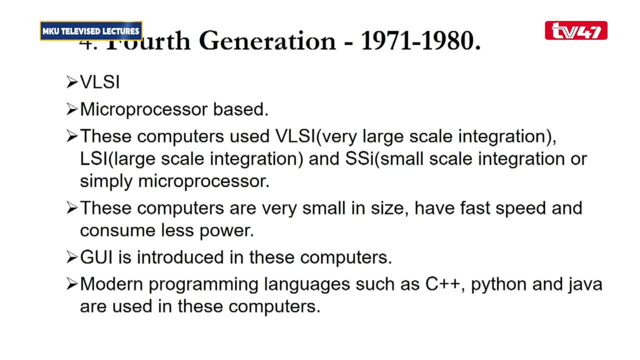 It was small in size and the speed of those computers was quite higher. They used a graphical user interface Where the users could easily work with them. they were more user-friendly and they were using a programming language and therefore users could even develop applications based. 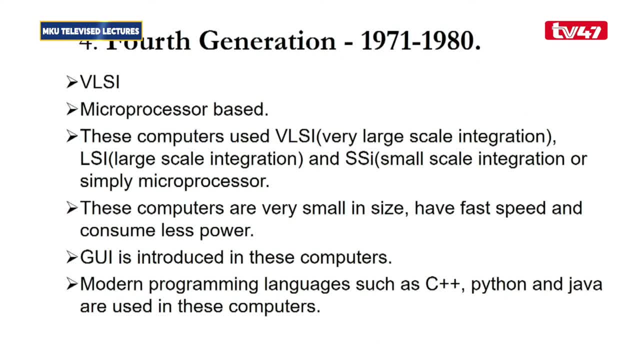 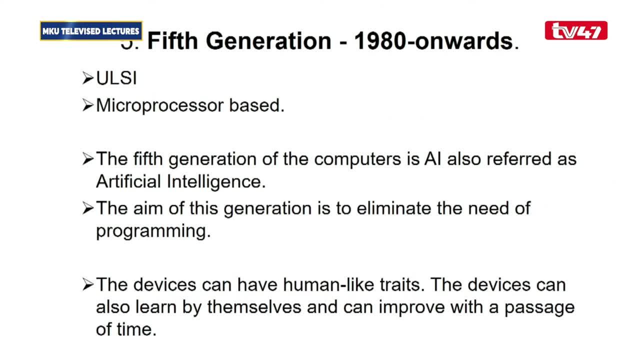 on these generational computers And the last generation is based on the fifth generation. The fifth generation is from 1980s up to current, or up to today, So this is based on ultra-large-scale integration. Ultra-large-scale integration: we started with integrated circuits, let's say hundreds. 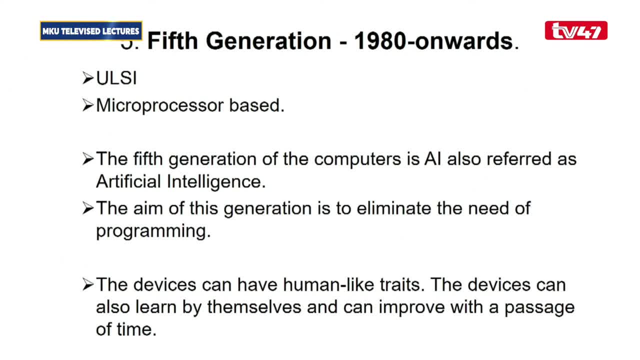 of components integrated together. Then very large integration of components, that is, thousands of components together, And here we are talking millions or billions of components integrated together into one single component. And what is happening again? the computer is becoming smaller and smaller in size and 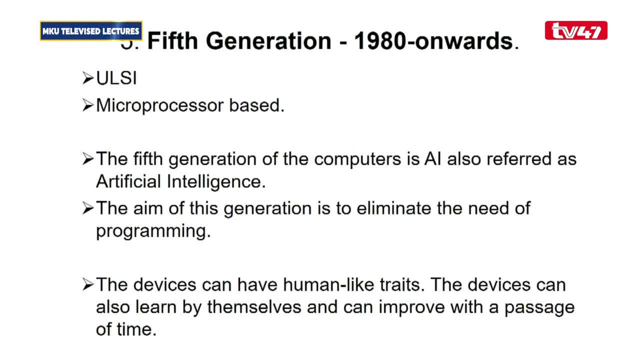 the performance is becoming much, much better. So this fifth generation. what's the key aspect of the fifth generation is to have a computer that is using the artificial intelligence or the use of programming language that makes the computer to behave like a human being. 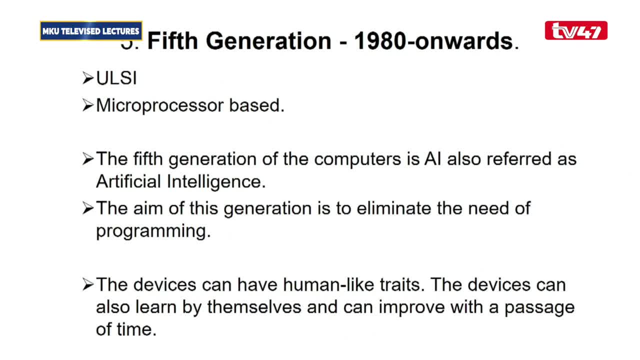 In other words, this particular generation which is still under development. it is not complete, because this is the current generation that we are in. When this generation is complete, we are expecting a computer that would behave like a human being, In other words, in terms of the operation. 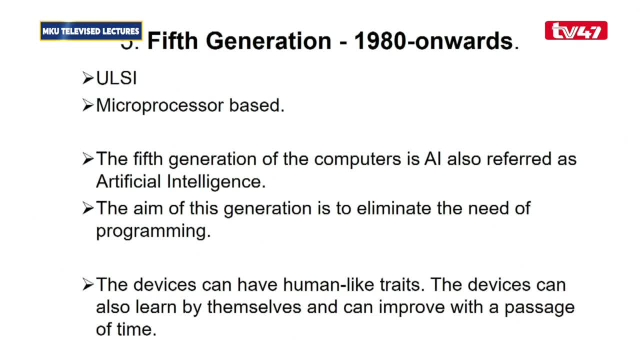 The current computers that we are using nowadays you enter the command by typing, where the characters appear on the screen as you type, so they take input through the user command. But in this case, how does, when you say they'll behave like a human being, human being they? 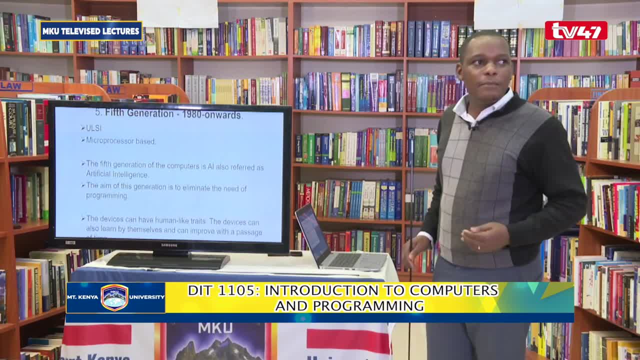 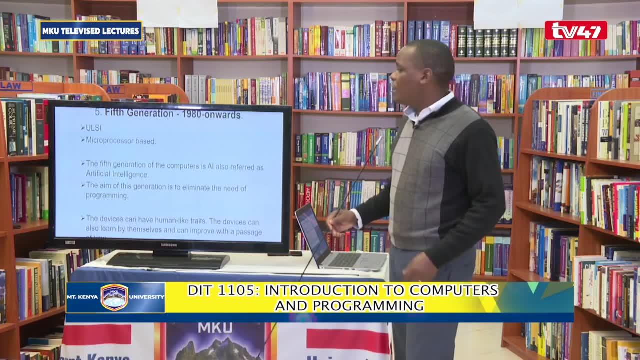 instruct. through the voice command, You tell a human being move from this point to this point. voice command And therefore this fifth generation will be taking voice command. So instead of typing, you'll be talking to a computer. you talk through the microphone. 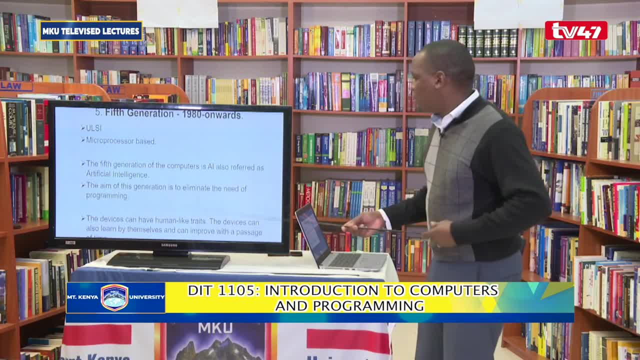 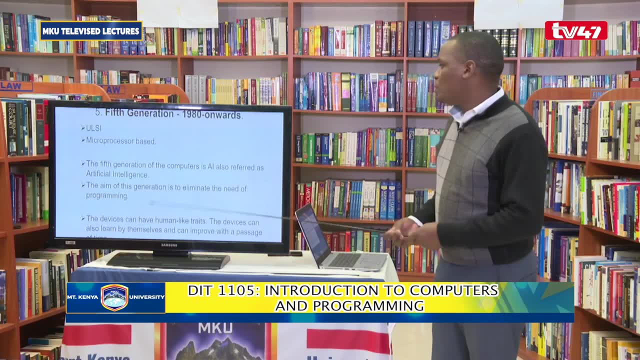 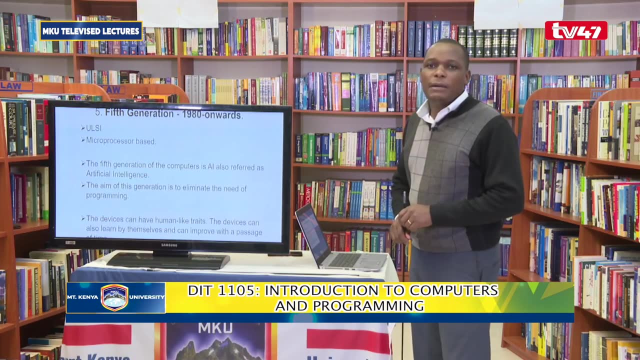 as the characters appear here on the screen. So they are based on artificial intelligence, or this generation will be based on artificial intelligence, which is going to assist in making even the functional Uh aspect of this computer to be much, much better. 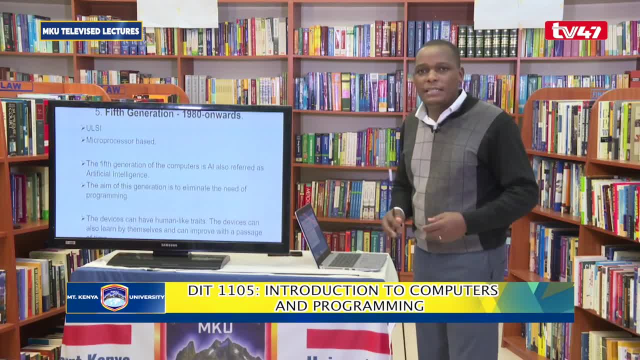 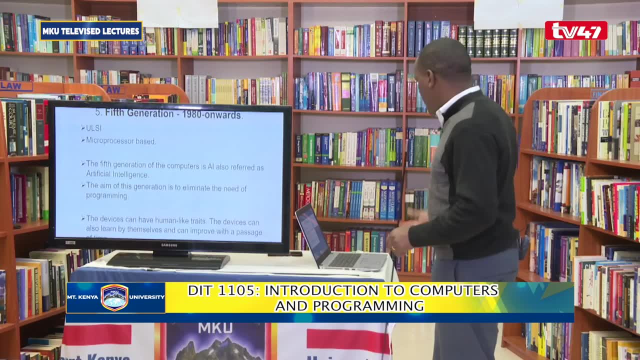 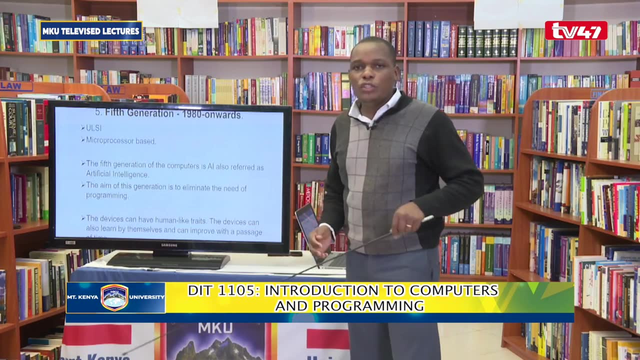 These are still in development. We have some devices that have already been produced, like in mobile phones, which are still taking voice command. like you're using a mobile phone, You have some contacts that have been saved in that mobile phone and maybe you want to. 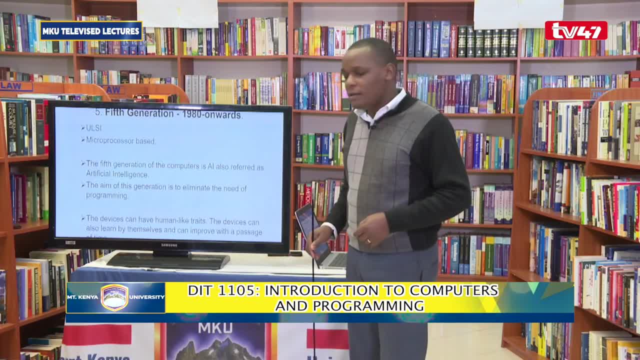 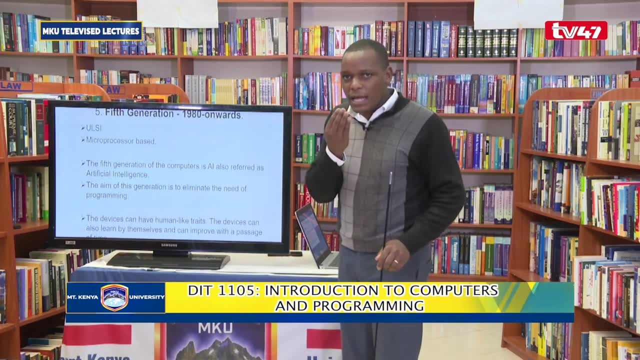 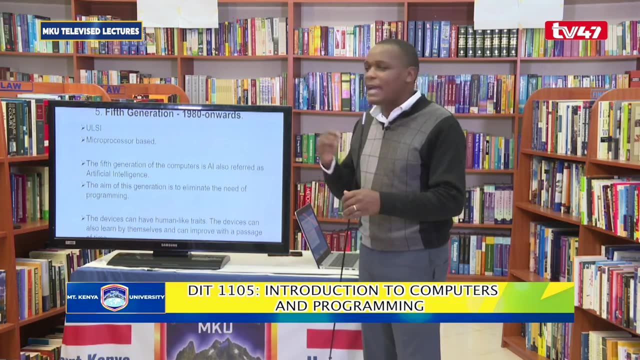 call or to dial a particular number by the name you have saved. This is somebody by the name Peter. Instead of scrolling down manually, you can just talk to your phone. say Peter, and the contact Peter appears on the front screen and you dial it directly. 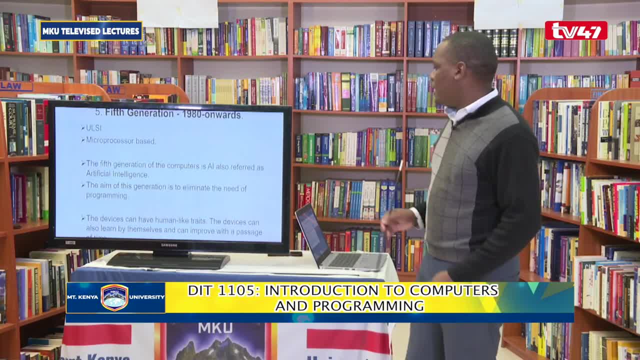 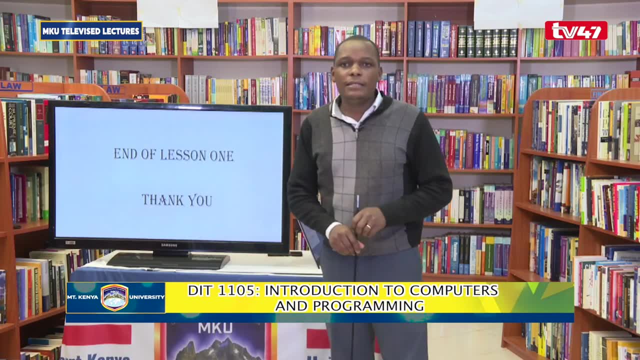 Therefore, this particular generation is still under development. So that brings us to the end of our today's lesson. Thank you. These televised lectures supplement our robust online learning going on on our app. We hope you have a great day, Thank you.